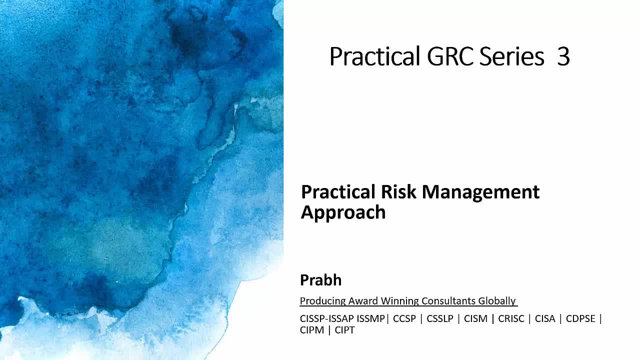 visibility how the enterprise risk management implement in the organization. So if you're new to the channel, do subscribe to the YouTube channel and click on the bell icon to make sure you should not miss my future videos on a similar topic, because I'm planning. 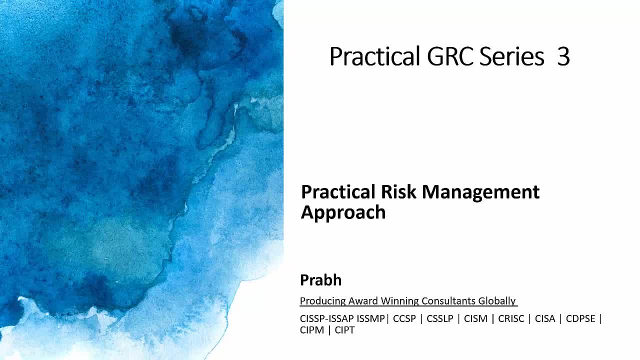 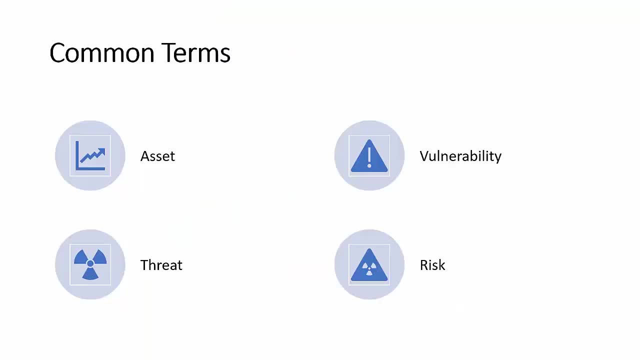 to make more and more practical videos on GRC, cybersecurity and network security and cloud. So, without wasting your time, let's start with the first part, Thank you. Before going to start about risk management in detail, we should know the basics first. 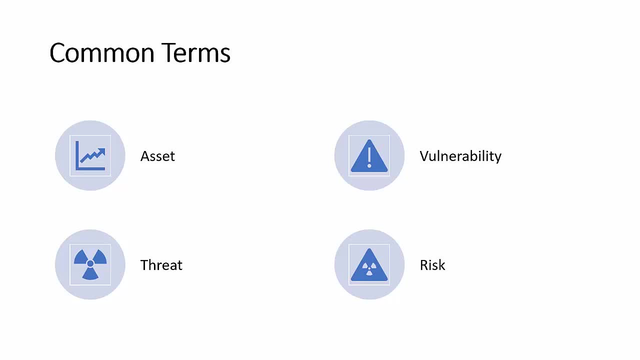 because until and unless you don't know the basics, you cannot be able to understand the risk management. So some basic terms are like, example: asset. Asset is anything which create value for an organization, And we have a two type of asset: One is called as a tangible and one is basically called as an intangible. 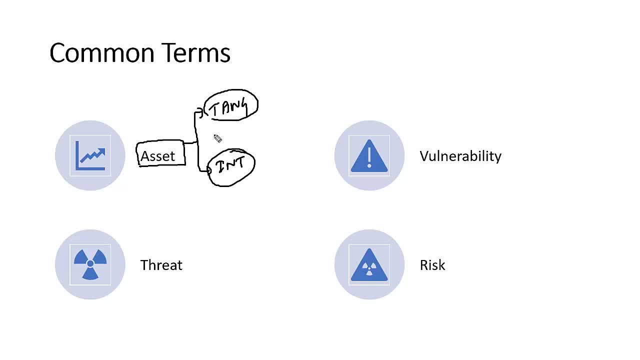 So when we're talking about tangible asset- anything which is physical assets- Intangible. Intangible is anything which is a logical asset. Let's take example: we have a server. Server is a physical asset which can touch, but the data in the server is an intangible. 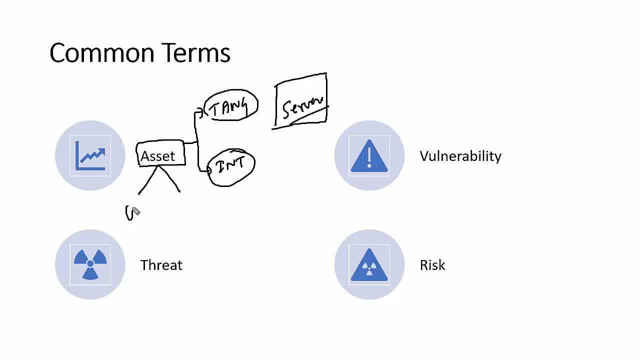 asset. Asset valuation is also two type. One is called as a qualitative and one is called as a quantitative. Qualitative is mapped with some reputation which cannot be measured easily, And quantitative is basically which is mapped with some monetary or numbers, like this asset. 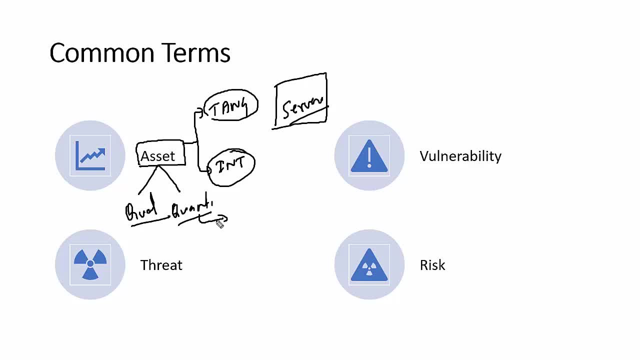 has a $7,000 value, $8,000 value and all that. So This is how you basically categorize assets. It's very important to know the value of the asset to perform the effective risk management, Because impact of the risk is directly correlate with the value of asset. 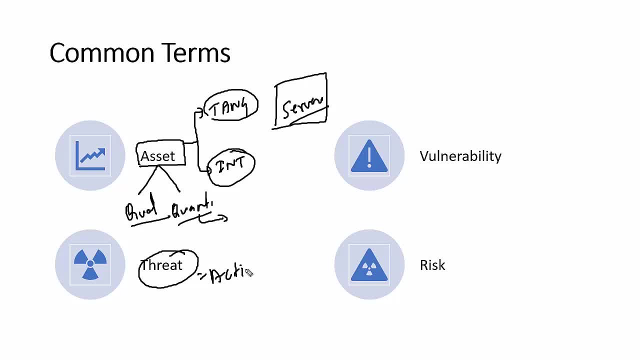 Second is basically called as a threat. Threat is an action that compromise the security. Okay, Threat is an action which basically invade the security. Vulnerability is called as a weakness that we have in the system. Let's take example: There is a hacker and there is a server. 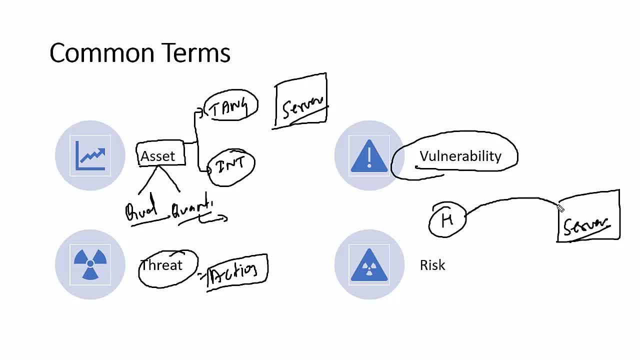 Hacker. Hacker trying to do attack on the server, And that is only possible when there is a weakness- Okay, in the server And he discovered the weaknesses. Some ports are open- Okay. some weak passwords are there- Okay. inappropriate functions and everything. 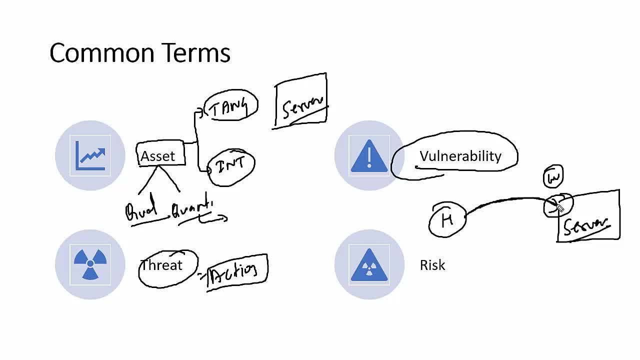 Okay, so he used the opportunity and by which he tried to exploit the server and by which he gained access to server and by which he gained access to the sensitive data, And that is basically the negative impact on the organization. It means some hacker hack into the system and there is a disclosure of a data and company. 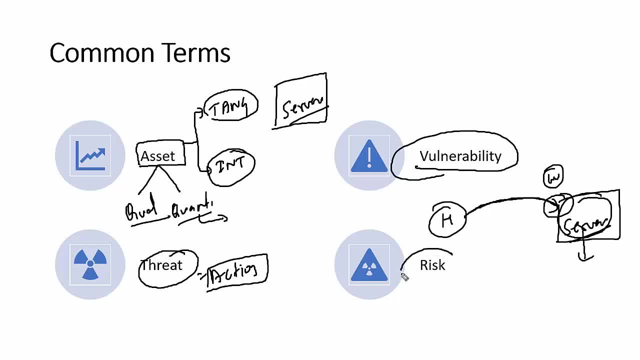 has to answer for that particular impact and that lead to the overall risk. Okay, So summary is that hacker is a threat, Vulnerability is called as a weak password And risk is the overall impact which company basically face. One more example is a ransomware attack. 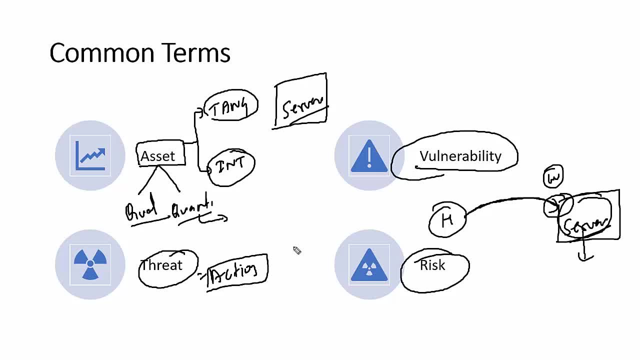 So there is a ransomware attack against the server. There's a ransomware attack against the server, So ransomware is a threat. They attack the server. They attack the server because they discover the weaknesses. There's no frequent backups is happening. 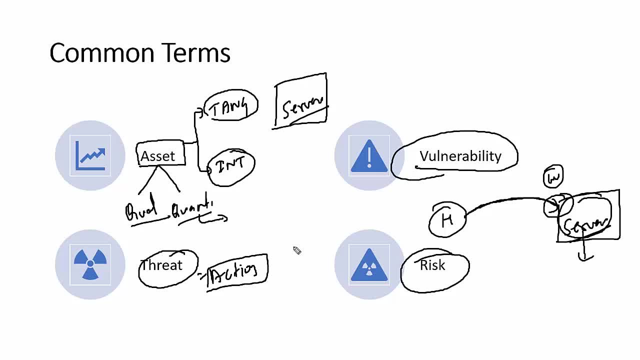 So they encrypt the data and now company unable to retrieve the data, company unable to decrypt the data, So that is a loss of an organization that is basically called as a risk. So it is very important for us to know this basic terminology before moving to the next. 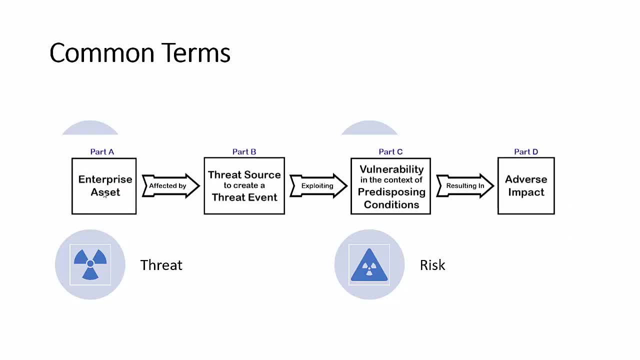 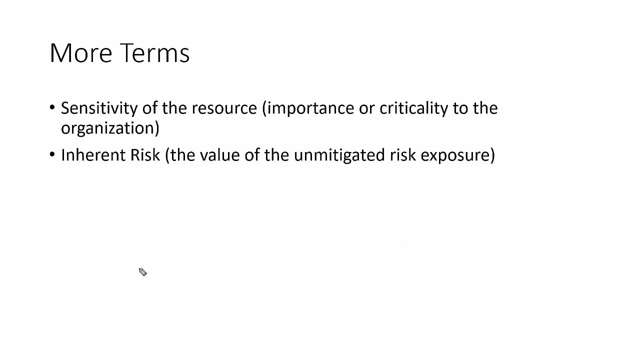 part- So I have one term here- is enterprise asset affected by the threat source which create a threat event, and that exploiting a vulnerability And that is basically result Into the adverse impact. Okay, So let's move to the next part. So it is basically a risk which is left, which is there without implementing control. example, 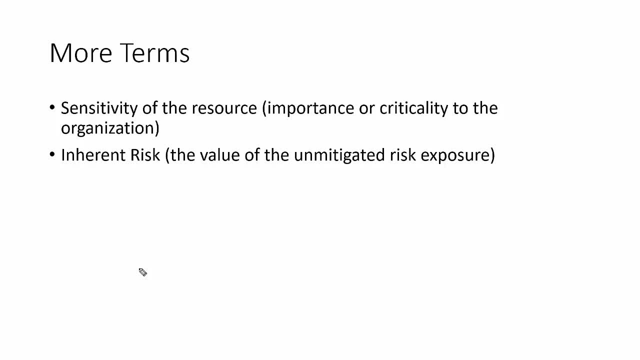 We know there's a thousand systems are there in the organization. Currently we don't have any controls in that we need to consider control, but we have. this concern is how to implement the controls. It is difficult for us to manage that traffic because we're receiving a huge amount of traffic. 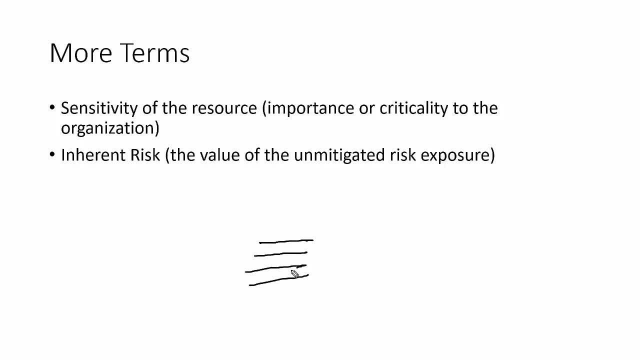 Okay. So example we're receiving right now for traffic. Okay, It is difficult for me to monitor, So something we have already accepted. there is an inherent risk because if I, even I, miss one packet, it might have some exploit which have a further system. 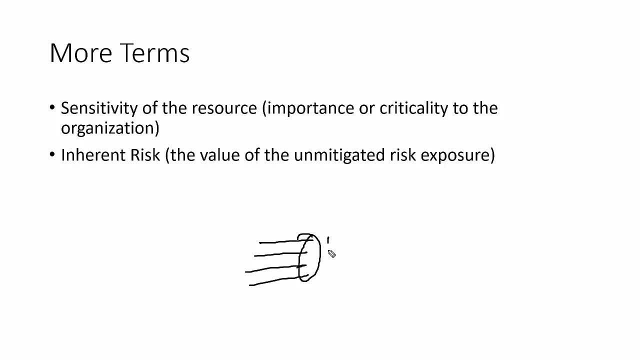 So currently there is no control for the risk. but now what happened? we installed some filtering solutions by which we can filter some of the traffic. So by this we can able to control only two and we left with other two, So these two are called, as a result, risk. 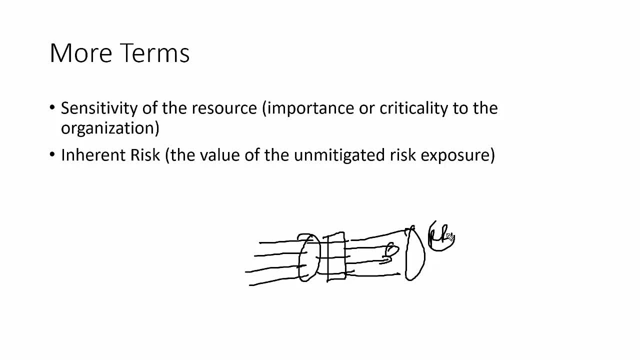 So risk before implementing control is an inherent risk. risk before untreated is called as an inherent risk. Okay, So after the treatment is called as a result risk. example- this is my inherent risk. We put a filter and after that we can able to limit to one particular traffic. 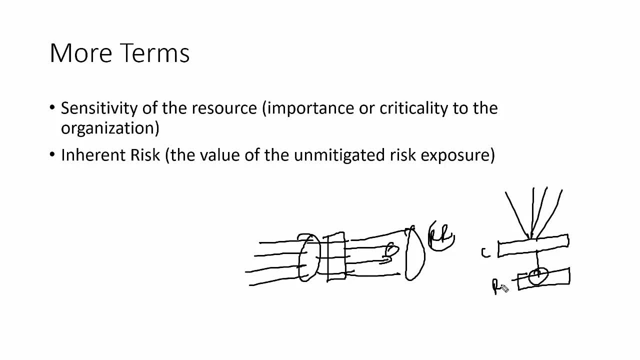 And this is the thing which is left after implementing control- that become a residual risk. Okay, So that is another important term We have. further to that, We also have a compensating control. The controls is basically introduced to reduce the impact, but we have this assumption: control. 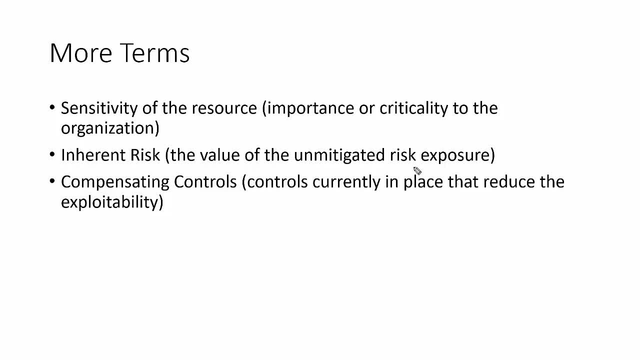 is introduced to reduce the impact, But primarily, control is introduced to reduce the impact. Okay, So this is the likelihood. actually, How Suppose this is my server? okay, server one and server two. So now what happened is- let's take an example of- there is an attack where it's sending. 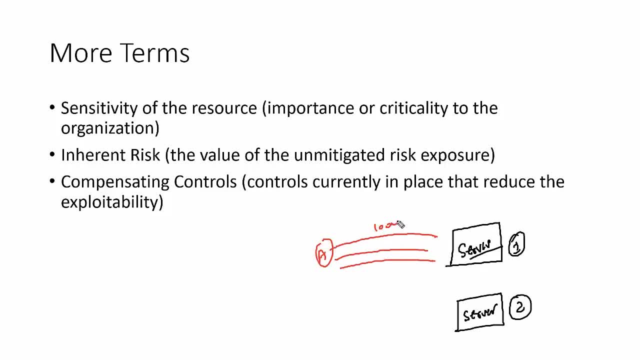 a hundred traffic, a hundred packets, thousand packets. here also we're sending a thousand packets Now if in both side, in both server we don't have any control. So all the hundred servers, all the hundred packets are basically targeting directly on. 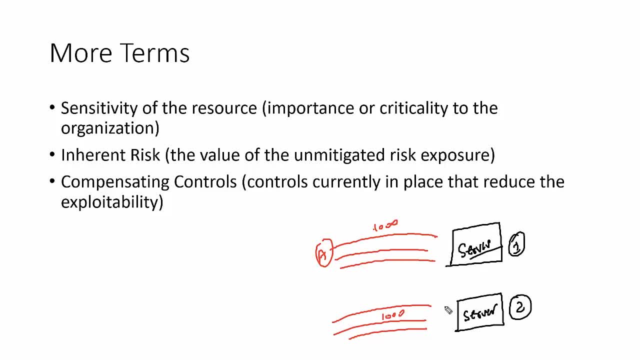 the server, which increase the load on the server while processing, and same applicable in the two. Now, what we did? we basically introduced the control, and this is basically called as a control. we introduce So by which what happened? We reduce a likelihood. 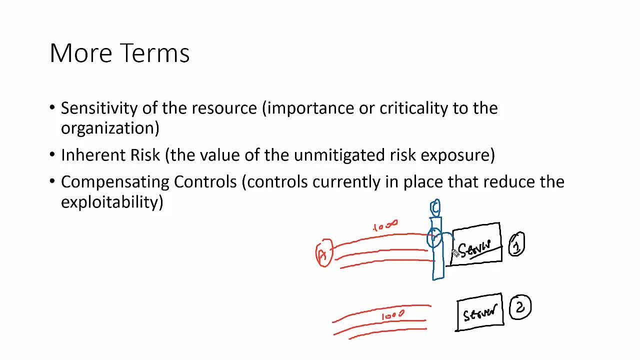 When we reduce a likelihood of traffic, it basically also reduce the level of impact. Okay, So control is introduced to reduce the likelihood. Okay, Okay, So control reduce likelihood. One more example: If my Gmail is only protected with the password, there is a higher chance that it can be exploited. 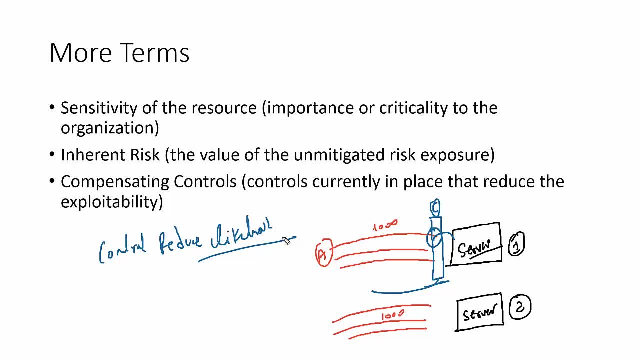 easily. But if Gmail is configured with the two factor authentication, the likelihood of performing the attack will be less Okay. Same with capture. also Without capture, there is a possibility of the bots. multiple bots can be attempt. But if I enable the capture by which I can delay the bots by which I can have a delay, 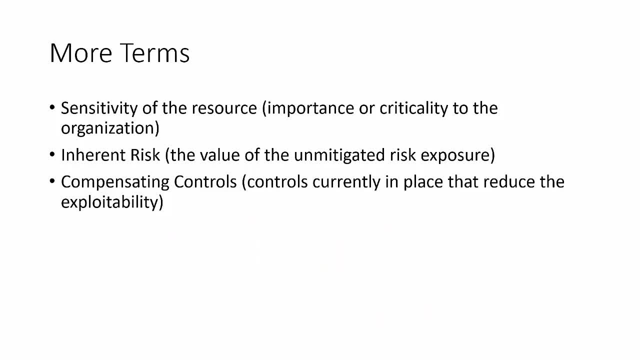 of the impact. So control is primarily introduced to reduce the likelihood. Okay, Then the risk which is left after implementing control. that is called as a threshold risk, And most of the cases, threshold risk is the one we basically accept. Okay, 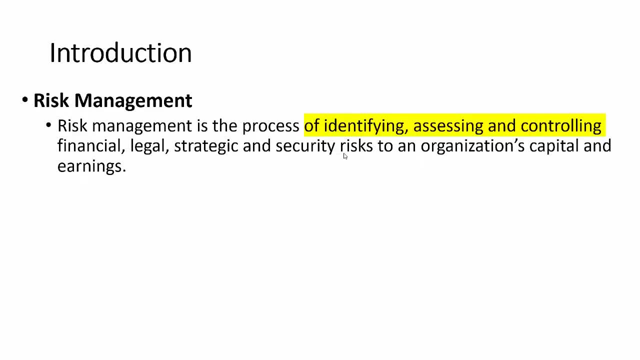 So, when we going by the definition of risk management, risk management is a process of identifying, assessing and controlling the financial, legal, strategic and security risk in an organization- capital and earnings. So ultimate goal of the risk management is to reduce the risk. 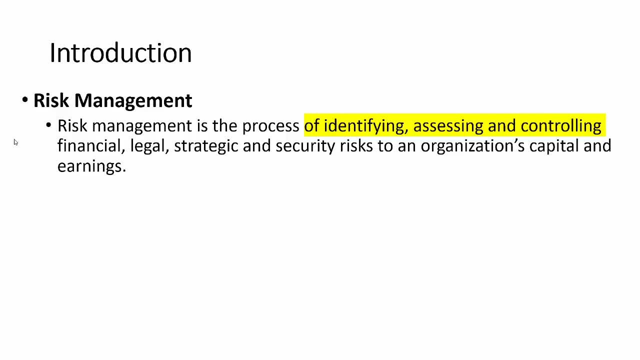 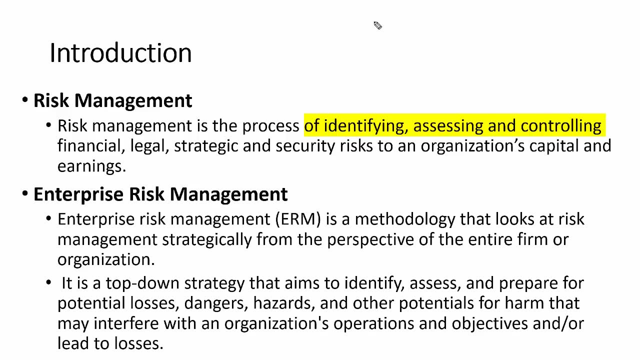 Okay, To reduce the risk to an acceptable level. So we have a dimension which is talk about in the organization which is called as an enterprise risk management. Okay, So see it right now. my channel is primarily on the information security. 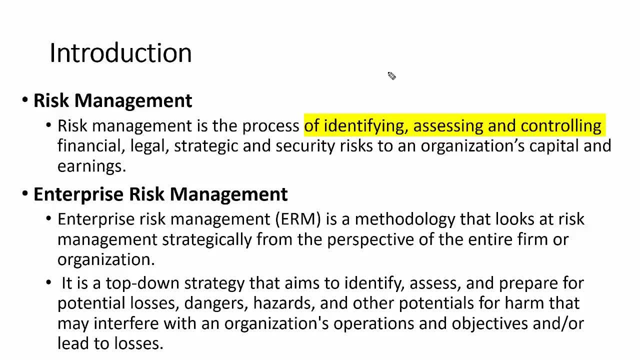 So I'm more. I'm talking about the information security, but we also have other dimension and same applicable in the case of risk management. In risk management, one risk management- we talk about information security risk management And one risk management is basically called as an enterprise risk management. 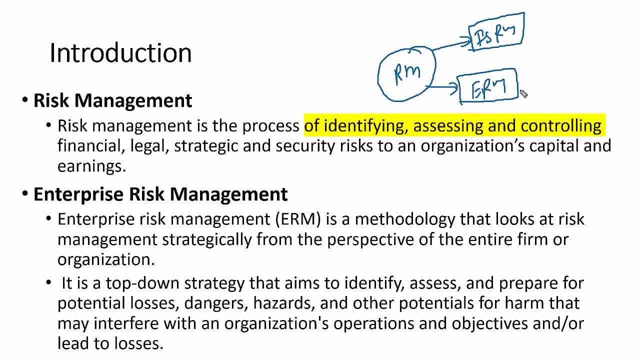 Okay, And this video is actually talk about enterprise risk management, which which covered the information security risk management. It covered the financial risk management. It basically cover process risk assessment and it also cover the regulator risk management. So thin line difference between the ERM and ISRM is ISRM is basically focused on the impact. 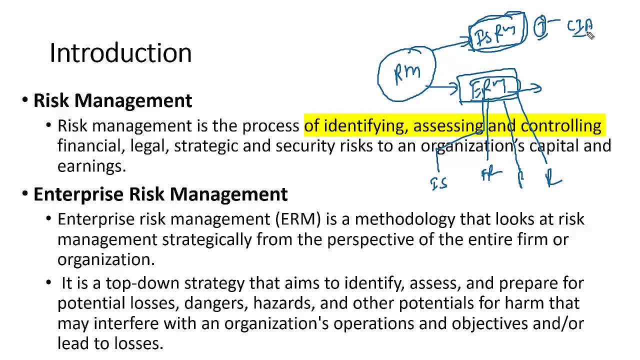 which map with CIA. It mean if there is a data get hacked by the server, what is the impact? So impact is map with CIA. Where's the enterprise risk management? It's talk about more holistic idea. If the server is basically down, the impact is basically on the customer. 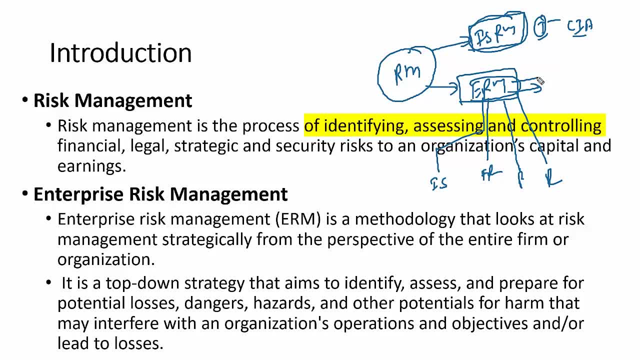 We might lose $7,000.. So here the impact. we're talking about more from the finance point of view. impact: we're talking about more from a business point of view. So enterprise risk management is a holistic approach which cover all kinds of risk management. 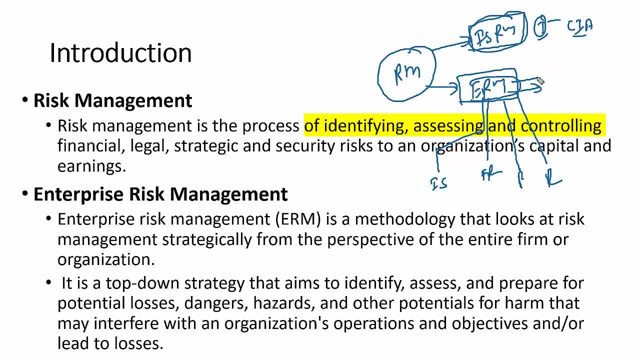 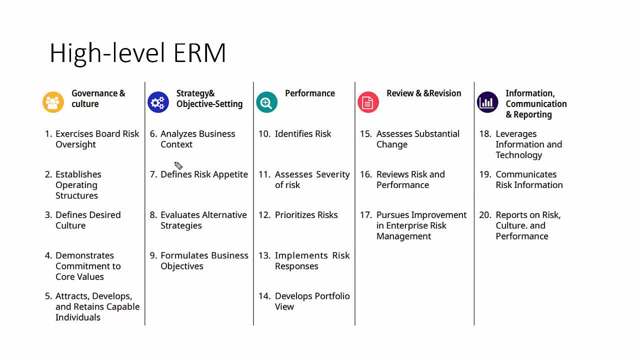 Even the CISO in some companies report to CRO. So CRO chief risk officer is responsible for the enterprise risk management, where the CISO is responsible for the information security risk management. Okay, So let's move to the next topic. So if you're planning to implement enterprise risk management in the organization, we basically 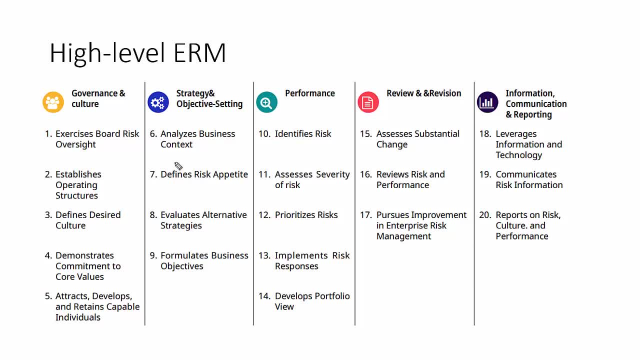 follow this approach. Actually, this is a reference of COSO. COSO is a framework which talk about how to implement enterprise risk management in the organization. So I have taken a small view of this particular COSO, but I'm going to discuss more in detail. 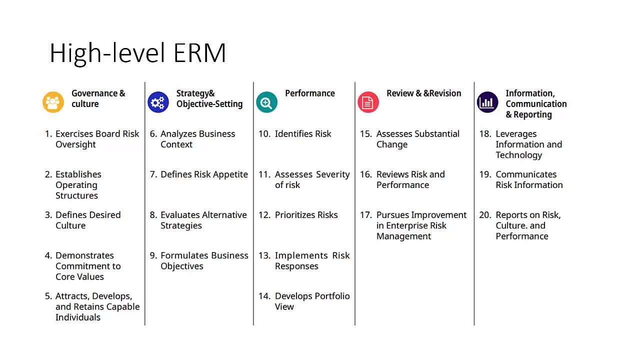 about the practical aspects, Okay. So here you can see. So the first step is exercise the board and risk oversight. it is very important to form the committee, Okay, Because that is how we'll drive the risk management. Then second is we establish the operating structure, how we're going to work. 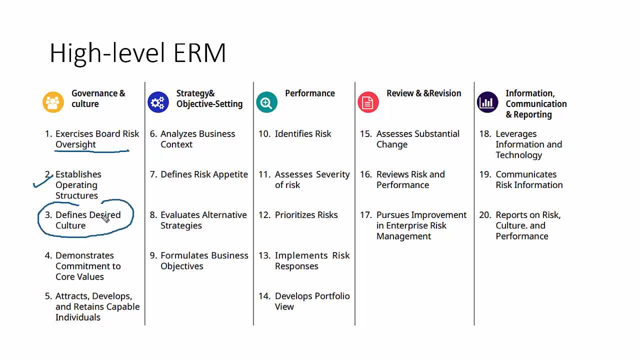 Then we need to define the desire culture. what is the defined culture we have? And then we talk about the commitment value toward the risk And all these things will publish in our enterprise risk management policy like: what is our value? what is the structure operating structures? 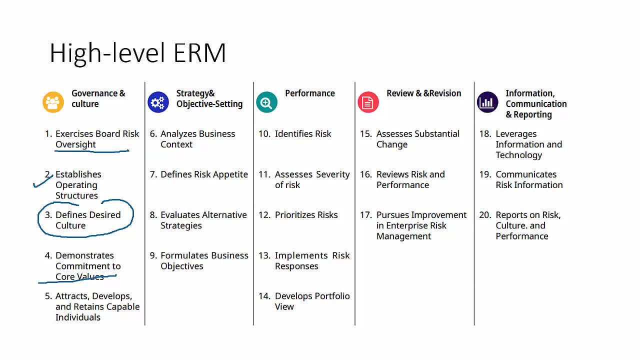 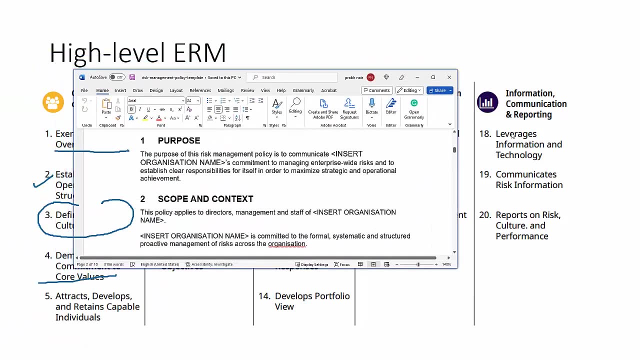 So it is very important. We need to create, We need to define the enterprise risk management policy in the organization, how the policy look like. Let me show you that. So this is how the policy look like. If you can see in the policy, the first part, we do define the purpose here. 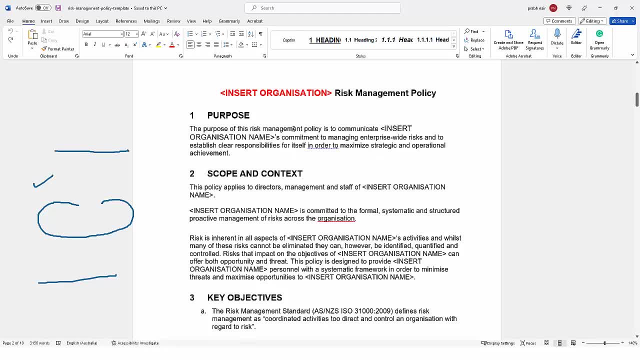 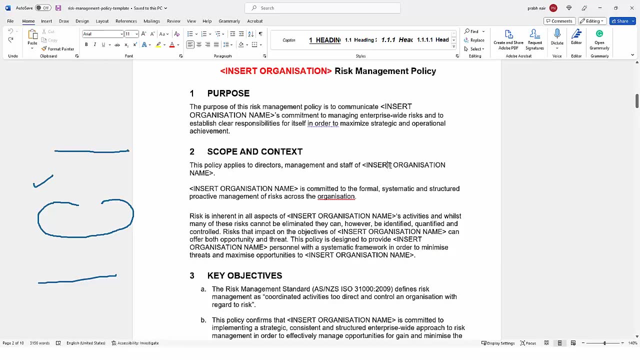 You can add a organization name. Suppose the purpose of the risk management policy is to communicate infosec, train or Aspen technology commitment To managing the enterprise wide risk, Then what is the scope of the policy? Like this policy applied to director management staff of our infosec, train or Aspen technology? 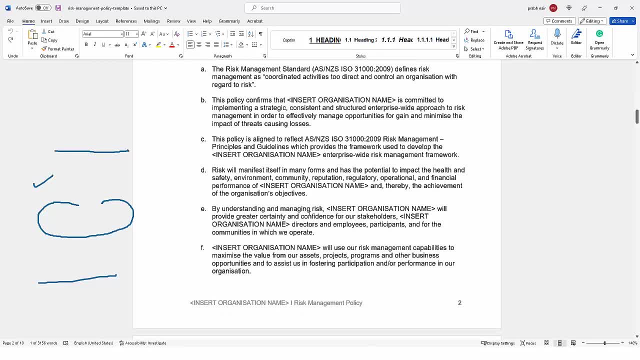 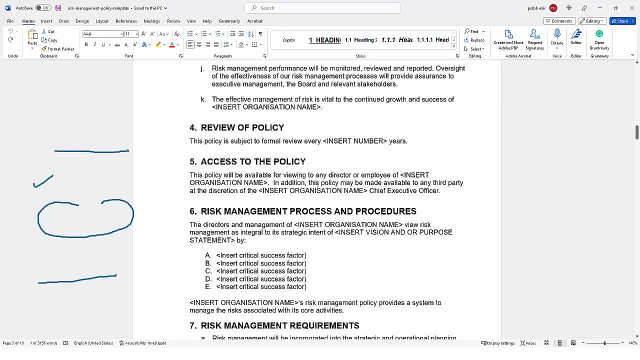 and committed to form the things. Then we talk about the key objectives we can add: Okay. Then we talk about review: when the policy need to be reviewed, What is the revision date? This policy will be accessible to whom? Then we describe the risk management process like identify, analyze, mitigate- here 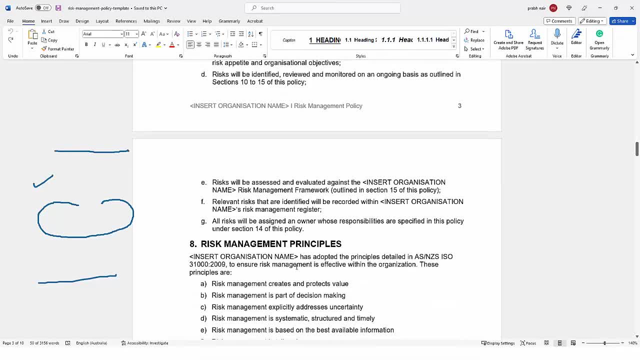 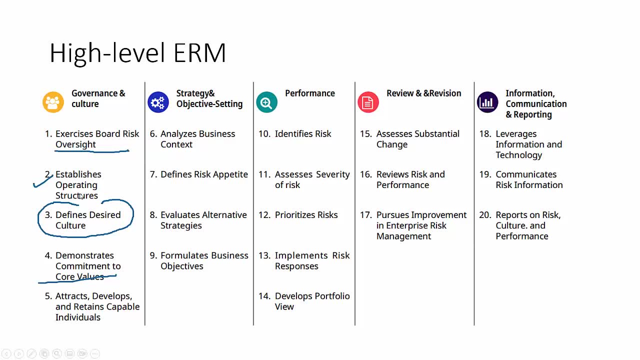 We need to document that. Then we talk about why are we doing a risk management? Okay, What are the principles we have? And then we explain the detailed process. So that's why everything which is part of a governance culture will be add in the policy. 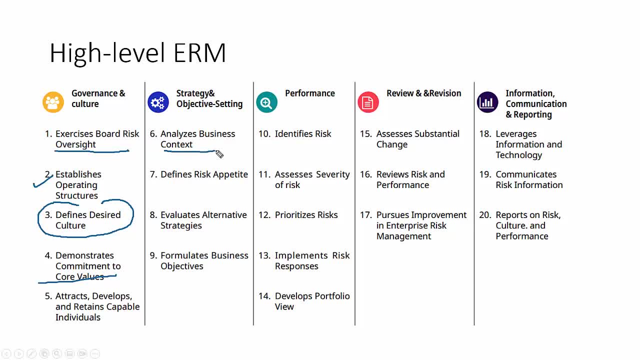 Then next important thing is called as a strategy objective, where we analyze the business context. Example: my business is basically doing the business of e-commerce, So availability is the most important thing. My business into healthcare, which is focused on the confidentiality. 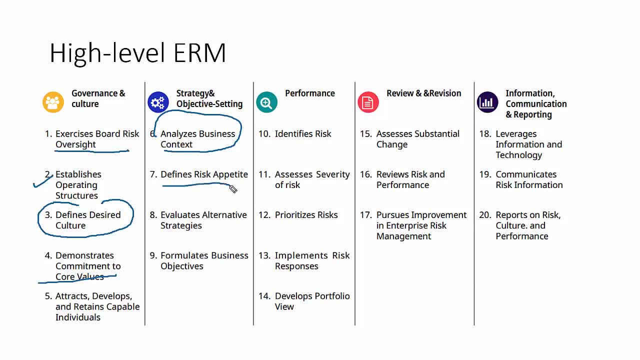 Then we define the risk appetite. In my further slide we want to discuss how to define risk appetite. Then we evaluate the strategy, We formulate the business objectives And then we introduce a matrix which is called identify, risk, assess, prioritize, implement. 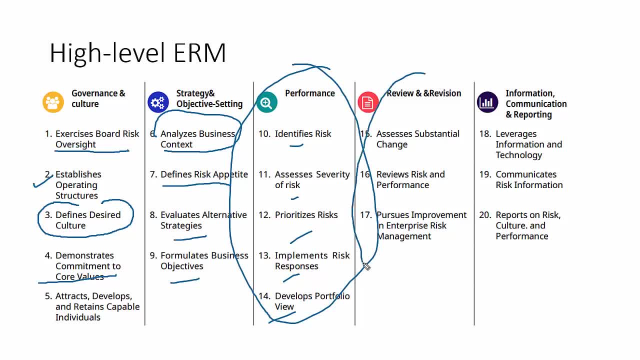 and develop. This is more like an operational level, And then we try to review and revision and then we communicate the overall culture to the people. So this is just a high level ERM, which is basically work. but don't worry, we're going. 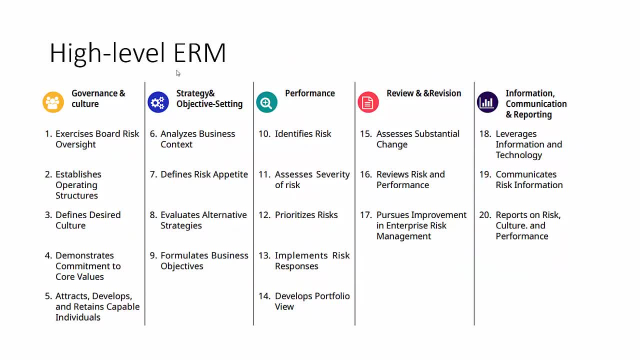 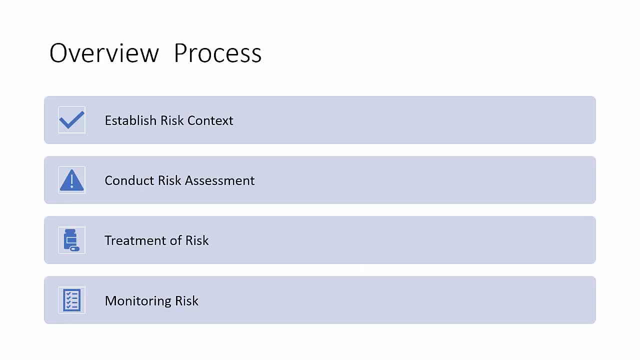 to discuss each and everything in a different way, in a more practical term. So, by end of the day, overall, if you see, the risk management, or enterprise risk management, is divided into four. Activity only first established, that is context. Second is conduct the risk assessment, which is on operational. 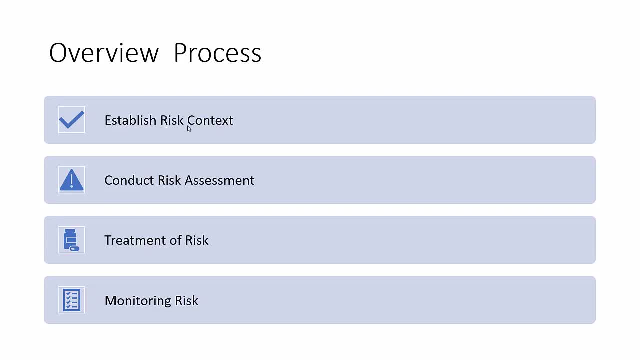 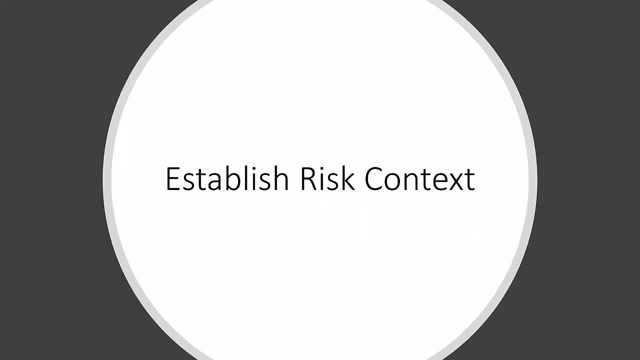 Then third is called as a treatment of the risk And finally we have a monitoring risk. Okay, So first part we're going to discuss is the stablish risk context. Okay, So next topic is called as established risk context. So when you're talking about risk context, it's all about the behavior and attitude that 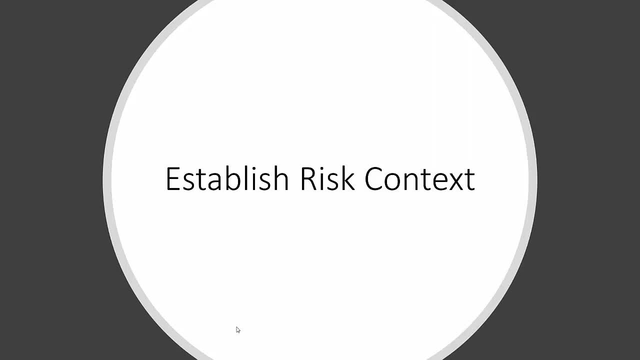 you take off a risk. from an organization point of view, It mean what is your attitude toward the risk, What is your perspective toward the risk, What is your risk capacity appetite? that is called as a risk context. So we have a two type of risk context, because it's very important to set the context. 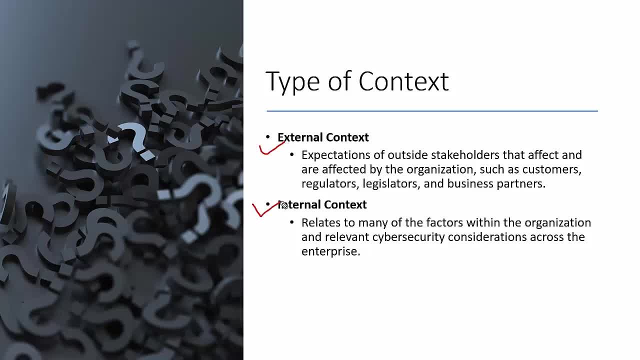 Okay, We have a two type of context. One is called external, stakeholder, and one is called as an internal context. So external context is basically mean what your perspective from a stakeholder point of view. you know, whatever the activity you're introducing, what will be the impact on the 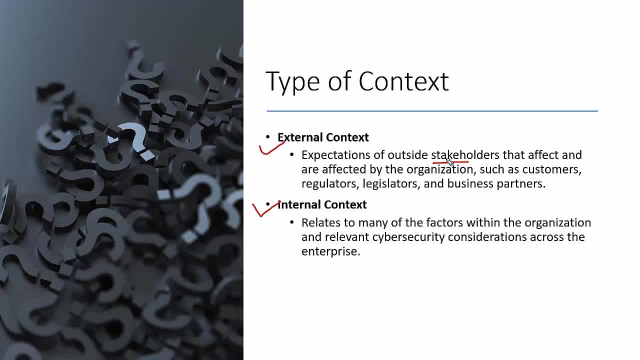 stakeholder with that particular activity. Let's take example: So far we were using some data and everything which is within a internal data centers, and all that. Now we move to the cloud. So what is the perspective? What would be the context? 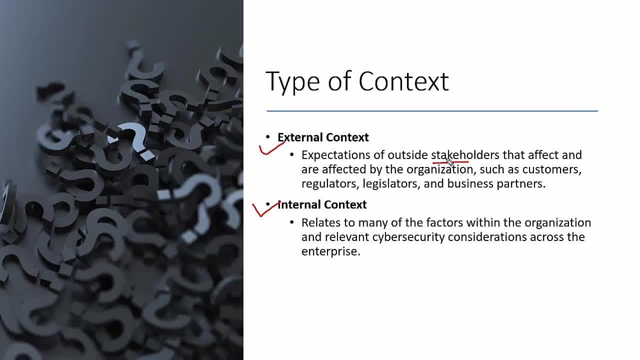 Okay, We have from a customer point of view, can we go for that call? We have some customer from Middle East. they are very reluctant for the cloud. So that is my external context, which impacts my behavior, which impacts my decisions. 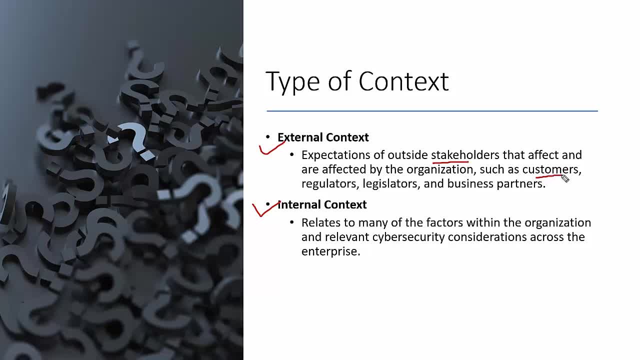 So stakeholders are there. Okay, Then we have a. customers are there. we have a regulators. they have legislatures and business partners. They have their own perspective about the organization and we should not take any kind of an action which impact their decisions. 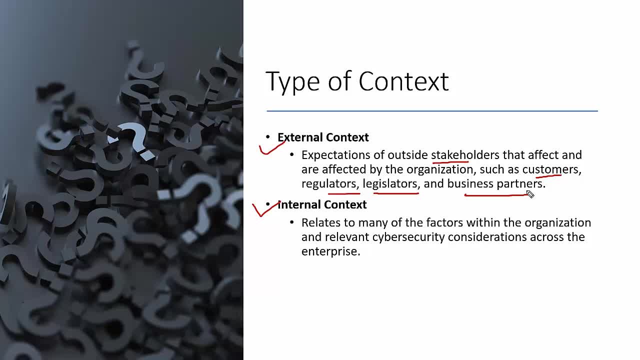 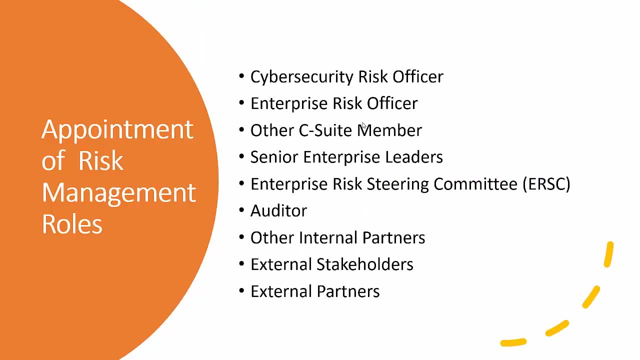 Second is called as an internal context. Internal context is related to many of the factors like which is happening within the organization. So whenever you establishing the risk management system in the organization, the first thing we need to set up the type of context. Once you have a type of context, we need to appoint some profiles. 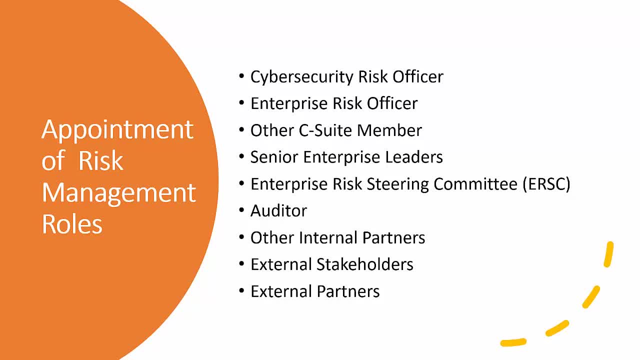 Okay, It's not necessary, You need to appoint all these people. But when it comes to the big companies, okay, we have some major roles, which is basically part of the risk management, like we have a cybersecurity officer. So when you take example of a cybersecurity officer in some companies, it is also called 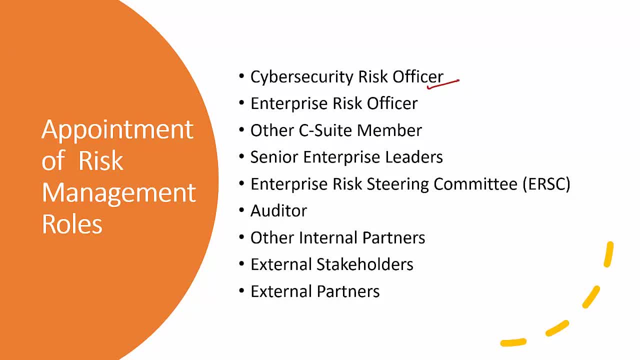 as a CISO, Okay, They are the one who manage the risk management process for our information system, And these individuals may also act as a risk owner for any particular risk in register or risk manager. So we have a risk manager who is designated by the risk owner, who remain accountable for. 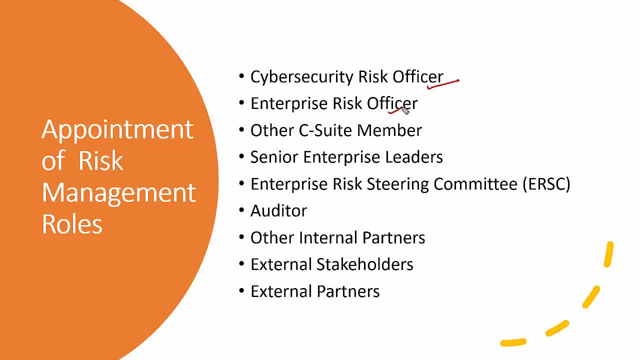 risk. Then we have an enterprise risk officer, a senior level person who accountable for managing and communicating a risk across the enterprise, And in some organization this position is also called as a CRO. Then we have other CISO members, like CIO is there. 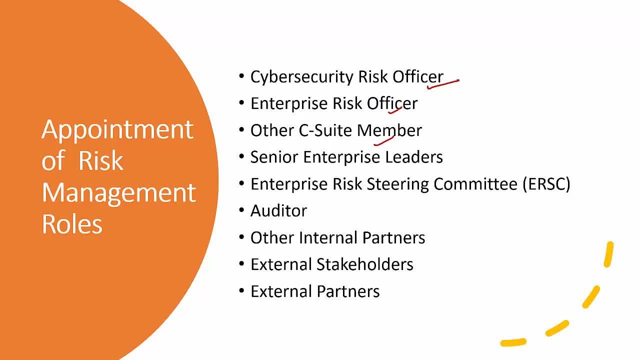 Then we have a CISO, We have a CPO, chief privacy officer and chief financial officer. Then we need some enterprise leaders. Enterprise leaders can be like: Okay, Okay. So enterprise leaders can be like: you have the agencies or corporate officials. 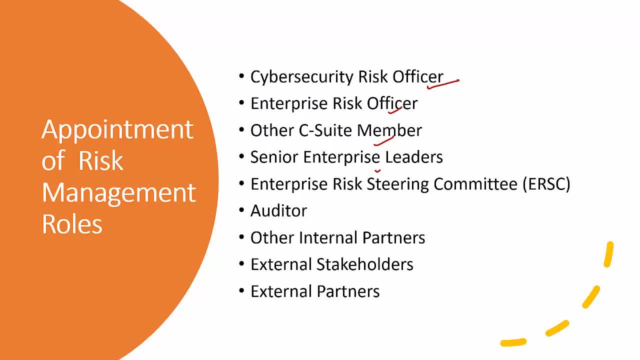 Okay, Who represent the various element of organizations, assist with managing and communicating risk throughout the enterprise. Then we also have an enterprise risk steering committee. They are the one who responsible for receiving a risk management information from throughout the enterprise And they're considering the overarching impact. 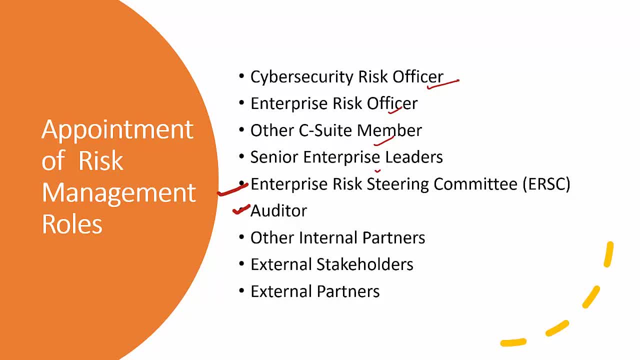 Then we have an auditor, which providing the independent verification regarding the achievements of the enterprise objectives. Okay, So they're in charge of the application of ERM process And they are the one who regularly report the issues and everything. Then we have internal partners. 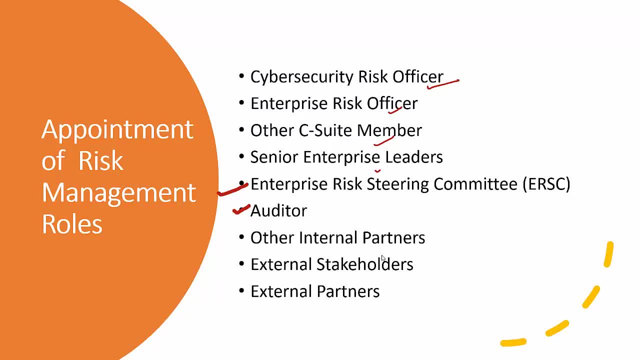 We have external partners, So we need to list down all these particular roles. Okay, So once you have these rules and you need to document that in your enterprise risk management policy, Okay, What are the roles we have? who basically carry the activity? 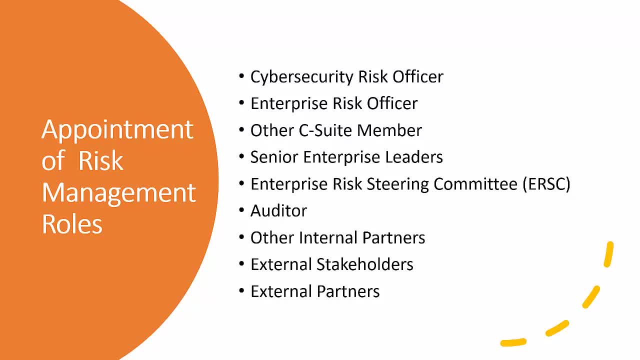 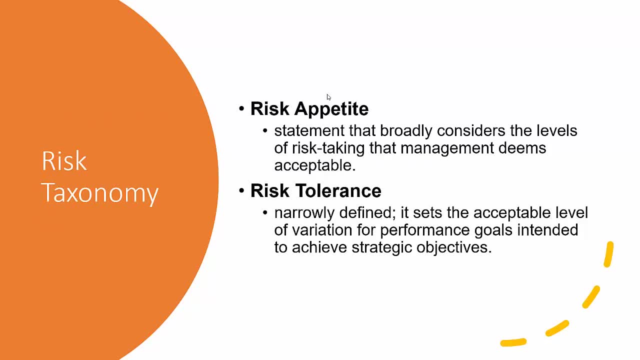 So that's the most important thing. So, once you basically, once you basically organize all the roles in a procedure document, which are the things that you need to do, Okay, the next thing we need to build is the risk appetite and risk tolerance. so if 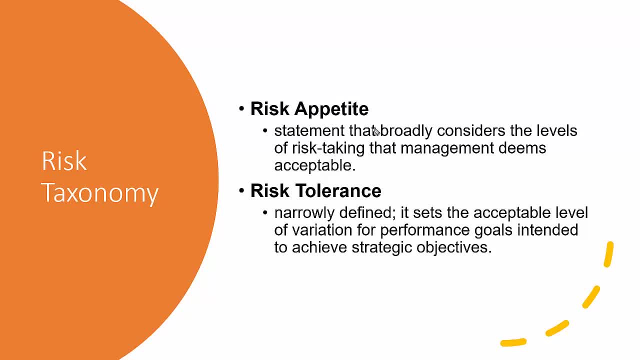 you go by the statement it's saying: risk appetite is a statement that that broadly described the level of risk taking the management deem acceptable, and this tolerance is narrowly defined, as said, the acceptable level of variation from performance goal intended to achieve the strategic objective. okay, so if you really want to know in a very basic num, let me give an best example. so, 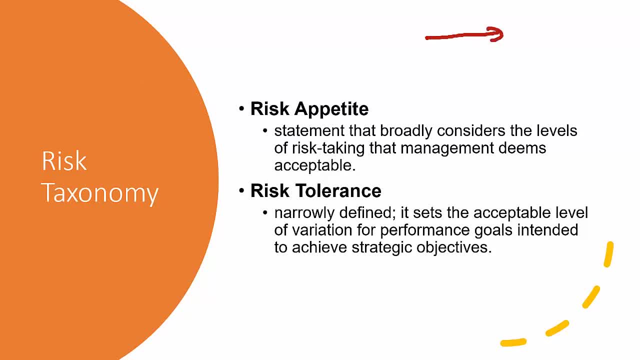 the salary which I am withdrawing every month. example. okay, the salary which I'm withdrawing every month is suppose $5,000, so this is the maximum investment I can do in a month. so this is basically my risk capacity. actually, I decided to spend five- a $1,000 from that in a mutual funds. so that is basically my 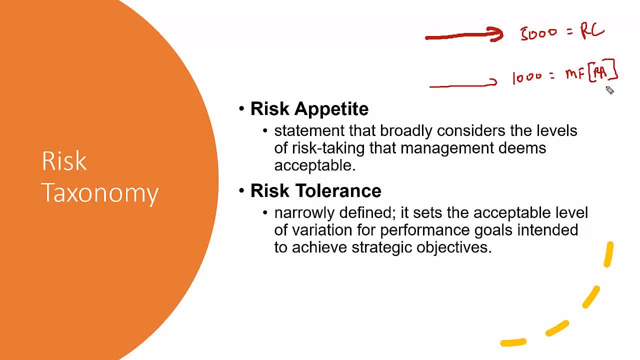 risk appetite. okay, that is basically my risk appetite. now I I can increase my appetite. okay, I can increase my appetite based on the market condition. so I understood: in one particular month I want to increase a mutual fund range and I went to 1200. so here there is a $200 of increment. I did 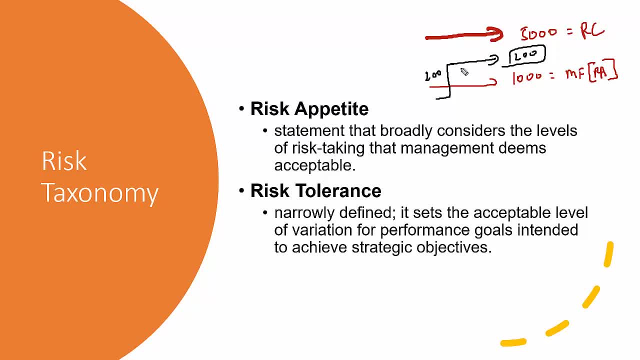 in my appetite because I found that month the market is great. this is basically my risk tolerance, or risk tolerance is always a deviation, okay. so one more example you can take: there's a State Department- okay, there's a State Department of Transportation, so they set the limit for its major highway. okay, so this can be. 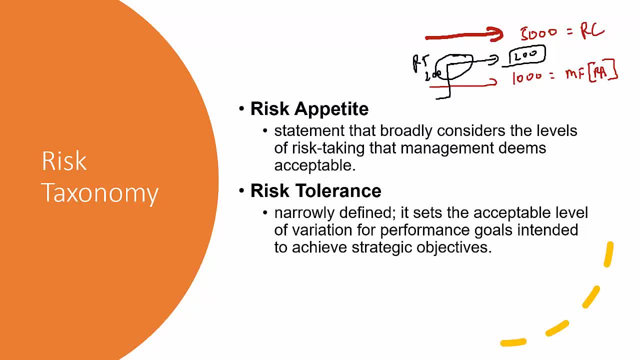 considered comparable to risk appetite. so it indicate that you know what the department executive believe is an appropriate balance between the traffic flow highway and environmental wear and tear and public safety. okay, so most drivers, however, will travel at the speed somewhat higher or lower than actual speed limit, rather than they obey the exact speed limit. so the point at 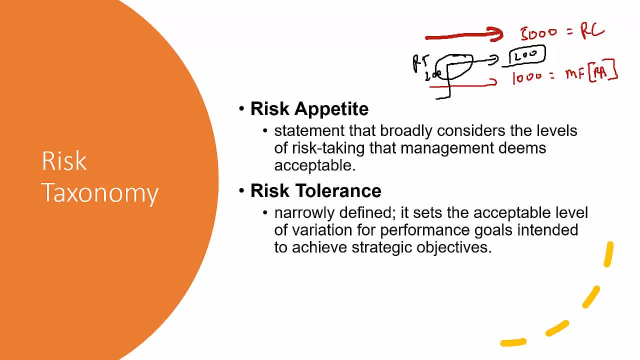 which law enforcement start to the ticket speeder can be view as analogous to the risk tolerance. okay, so the risk tolerance can be very so. you know, it's very important when you're creating a risk management policy and when you're creating a risk management system, it is very important to set the risk tolerance. 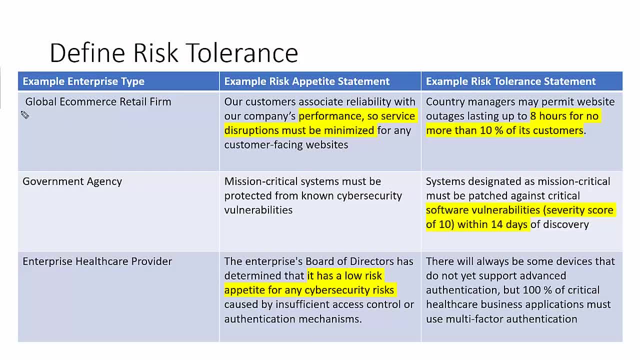 so we have some examples here. for the risk tolerance example, there is a global economic retail form we have, so this is the risk appetite statement for them. our customer associate reliability with our company performance or service reception must be minimized for any customer facing a website. so that is a. 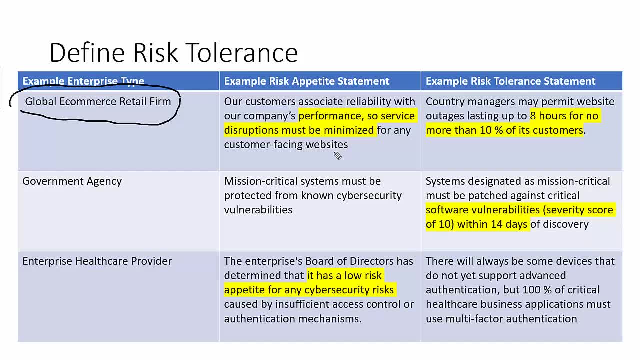 appetite for them, a level of risk they're willing to accept and they given the risk tolerance statement that country manager may permit website outage lasting for eight hours for no more than ten percent of it customer. based on this only, we will go for the risk tolerance entwickelt which will be around modo capture in the future, or any data set, the operating cost for a web site. attempt consumer some activity with El Pot, Lance, seguir deBox唱, denominar Talis et al. 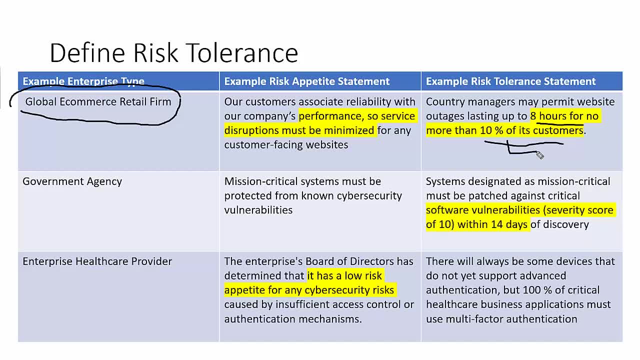 impact analysis. when you're calculating a risk right when you're providing a severity impact to the risk, during that time we consider this risk tolerance value okay. second example: we have a government agencies, so they have a risk effect. statement is: mission critical system must be protected from known. 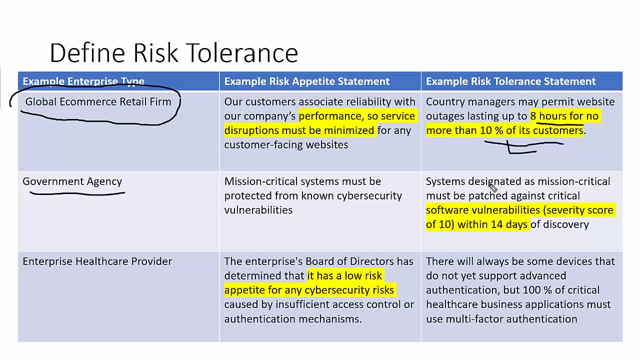 cyber security and vulnerability and we have said the risk tolerance system design as a mission critical must be patched against critical software vulnerability within the 14 days of discovery. so this is basically the tolerance we have. we can go above, but for that we need to take an approval. so 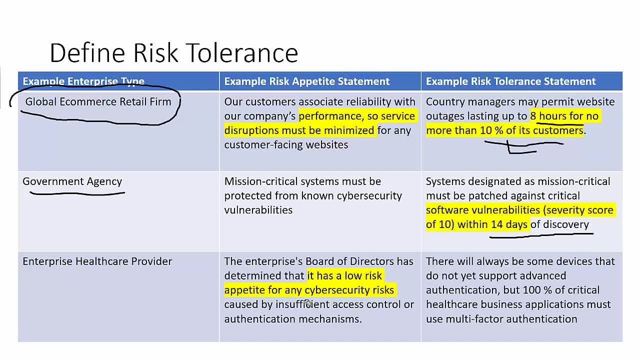 when I'm doing a risk assessment, I discover some of the vulnerabilities which cannot be patched in 15 days. so here what happened? this tolerance is increasing, so we need to see whether it how far it exceeding above the appetite and how much it reaching the capacity. so, based on that, we can take a decision. 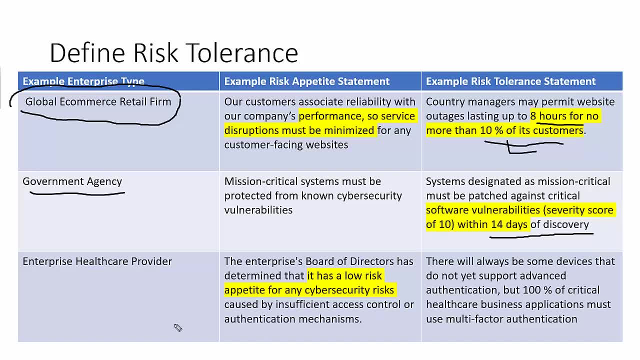 like, okay, we need to treat this risk or not? then third example we have: suppose you are working in the enterprise healthcare provider, so you have setting the policy. it's setting the appetite is enterprise board actor has their mind that it has a low risk appetite for any cyber security risk caused by. 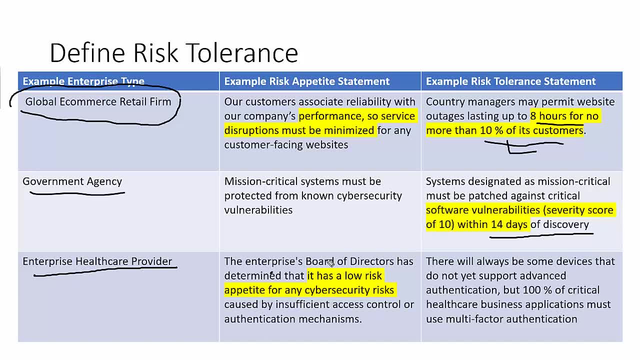 insufficient access control authentication mechanism. so we have said: there is tolerance. here is there. will we always be some device that do not yet support the Advanced authentication, but 100% of the critical healthcare business application must use multi-factor authentication. this is a tolerance level we have set, so if I discover any system without multi-factor, 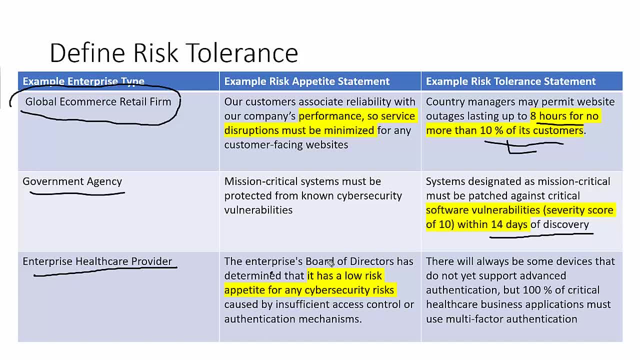 authentication. that is high risk. then I need to see the moreover impact rights over impact is basically that is a business application and it does does not have a multi-factor authentication. So it is very important in the initial stage set the tolerance If you are involved in seven business. 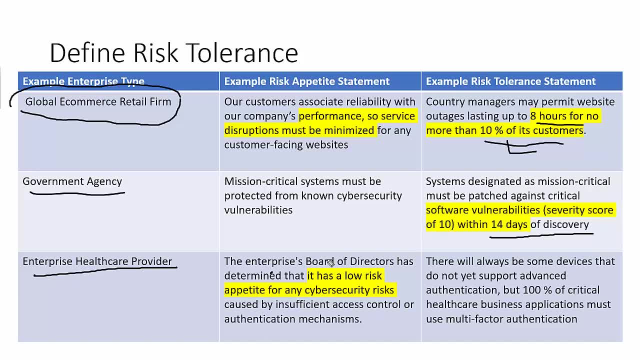 understand the seven business risk tolerance and who will be the best person to tell you about the risk tolerance? the business owner. Now there is a e-commerce firm. for them, availability is a top priority. There is a banking services. for them, confidentiality, integrity is the primary priority. 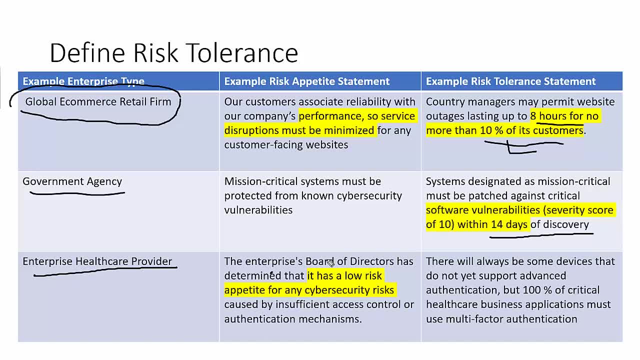 So understand their tolerance. Okay. so the one who running an e-commerce business: he's saying that okay, for 10 minutes I'm okay to accept downtime, because every minute I'm earning dollars, Every minute I'm earning million dollars. So for them, risk tolerance is basically 10%. 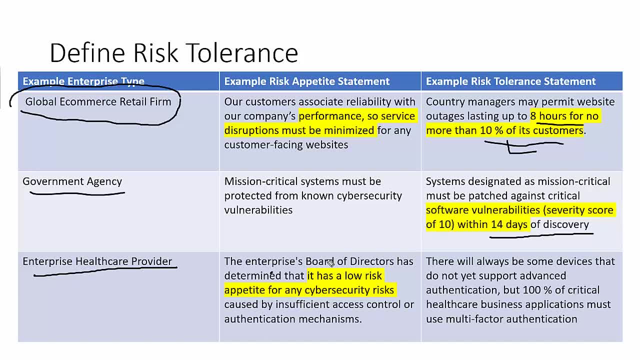 So, according to that, when I'm doing my risk assessment, I identify the impact is basically going to this level, which is map with the tolerance, or go beyond the tolerance. So that is why, in the initial stage itself, we basically set the tolerance. 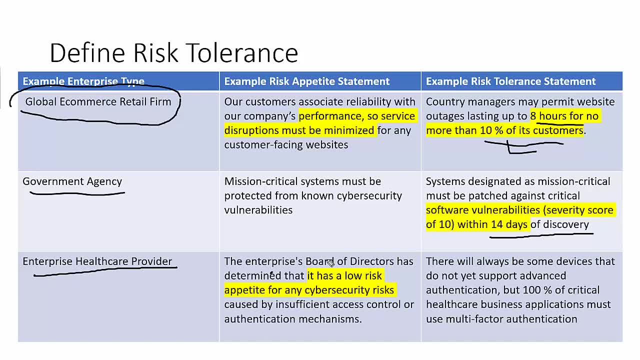 We spend a good amount of time. We spend good amount of meetings, spend great amount of time on the meetings with a business owner to understand exact risk tolerance. Okay so, because they are the final one who can tell you the tolerance level or tolerance functions of the business. 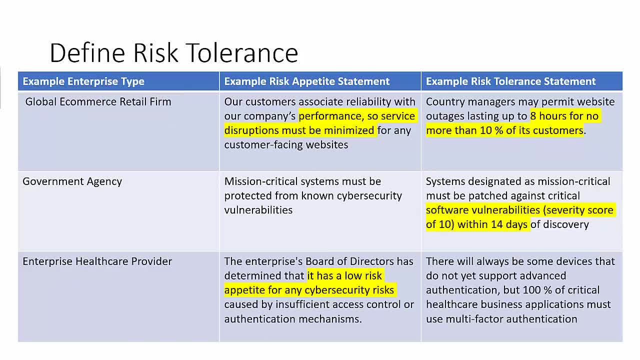 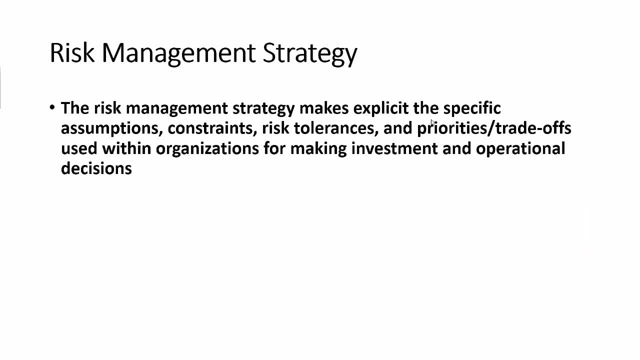 Okay. so it is very important for us to define. So, once you have this particular tolerance and all that, based on that you create a risk management strategy. So in a risk management strategy, you will explicitly specify the assumptions, You can define the constraints. 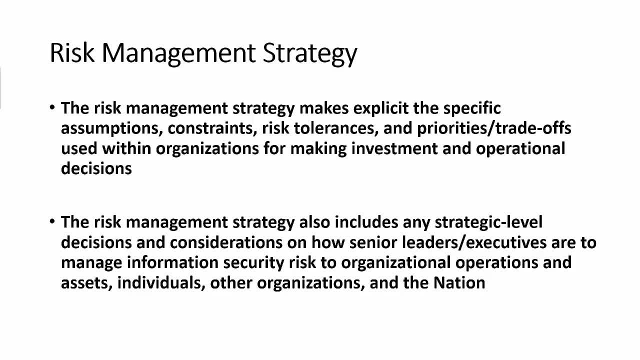 risk tolerance priorities- okay, And your risk management strategies include the strategic level decisions- Okay. so what will be the senior responsibilities, What is the responsibility of executives and how they're going to manage the risk in a day-to-day activity? So all these things part of the risk management strategy. 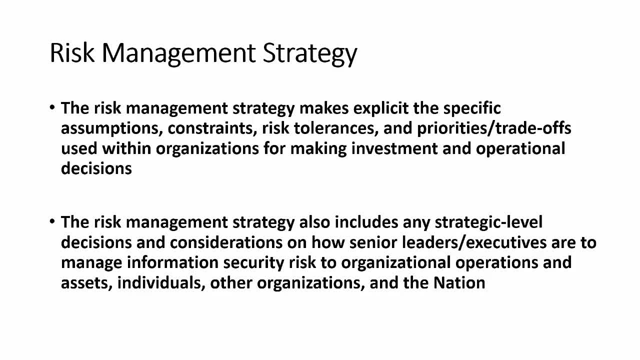 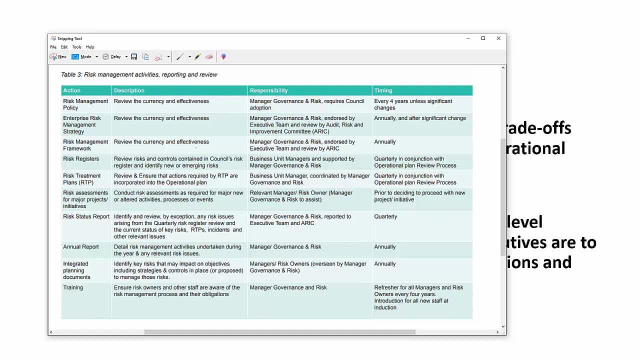 So I want to show you one sample So you get a better visibility how it works. So this is basically called as activities which we need to document in the enterprise risk management strategy. You can see that the first thing we need a policy. 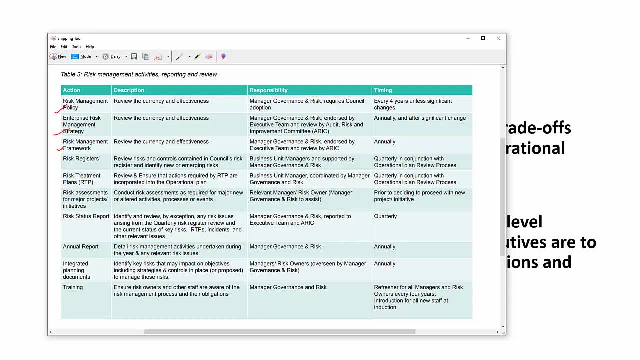 then we need a strategy. then strategy based on that we adopt the framework. then based on that, we document the risk. Okay, then we're creating a risk treatment plan. Then we have a risk assessment, risk status report, annual reports, integrate planning documents. 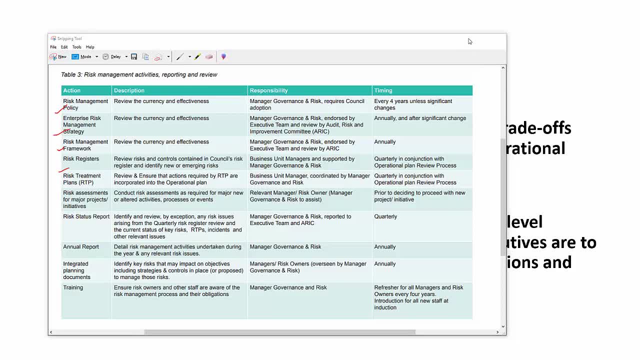 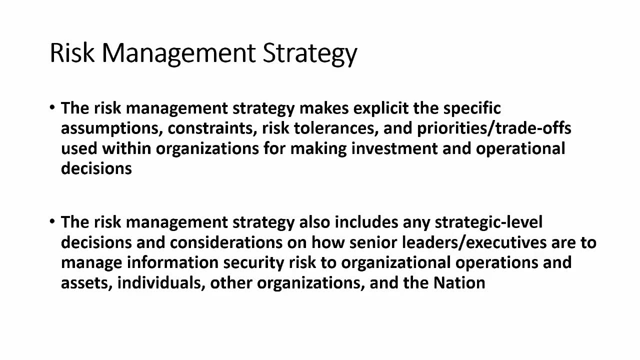 And finally, we have a training. So all these things is basically part of the strategy. Okay, all are basically part of the strategy document. So it gives you the high level idea about how things works and how activities has been implemented in the organization. 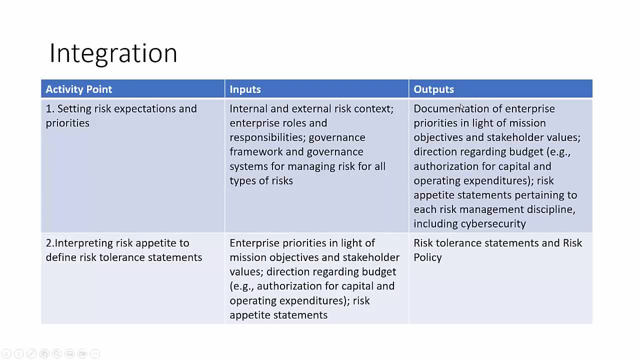 strategy is basically very important. so how we setting the risk expectation, that's a question, see, setting the risk expectation, setting a risk expectation priority is the most important thing. okay, so what is the input? we need an input from the internal, external context. we need a roles, we need responsibilities. 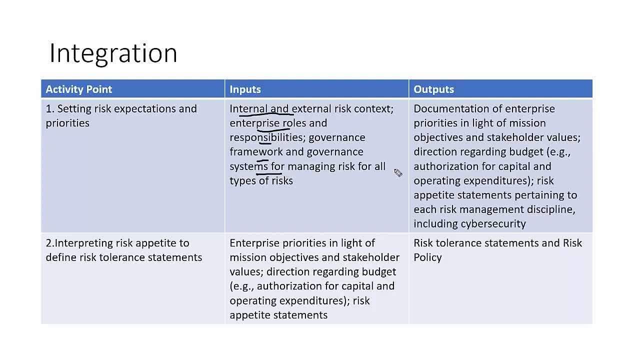 we need to know the frameworks. so this something is an input we have and what is the output like? we are documenting the enterprise priorities about the mission objectives. we need to know the stakeholder values from budget point of view. we need a risk appetite statement. okay, we need a discipline, functions and 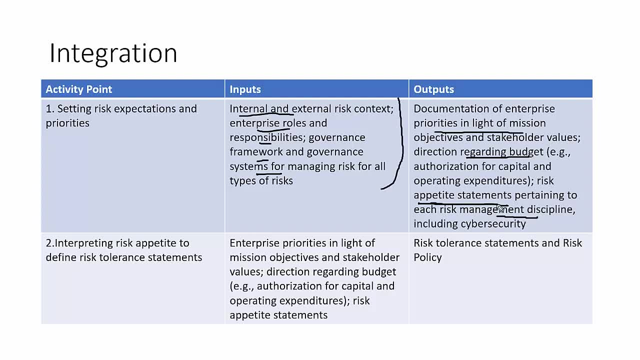 everything. so here, after understanding a context, we able to creating appetite. and then, once you have an appetite, you're going to interpret the risk appetite to define the risk tolerance statement. okay, so $1,000 is my budget for mutual fund. so what is the tolerance below or above? so enterprise priorities in light of a 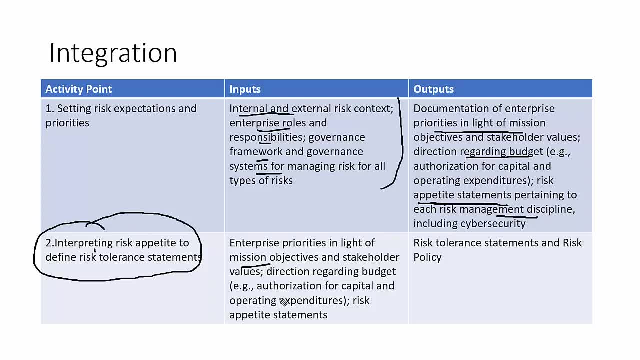 mission objective: stakeholders: okay, risk appetite statement. we build a risk appetite statement. we build a risk appetite statement, we build a. so that is the input and based on that, we create the complete risk tolerance statement and risk policy. so that is something is basically most important. so we need to collect all the documents, okay, and based on that, we create a. 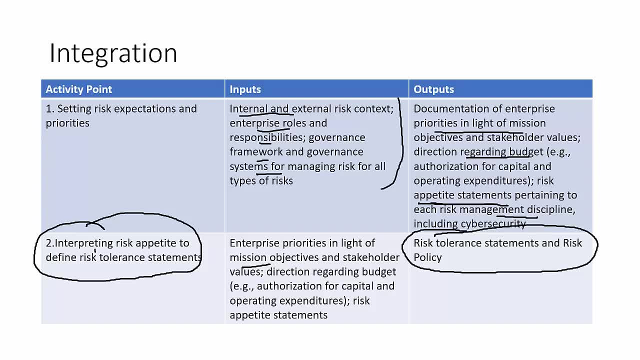 policy, we create appetite and, based on the appetite, we basically creating a risk tolerance statement and risk policy. okay, so that is what we need now. there's always a question arise about how to set a risk threshold, okay, how to determine the tolerable range, so I have a formula for that, which. 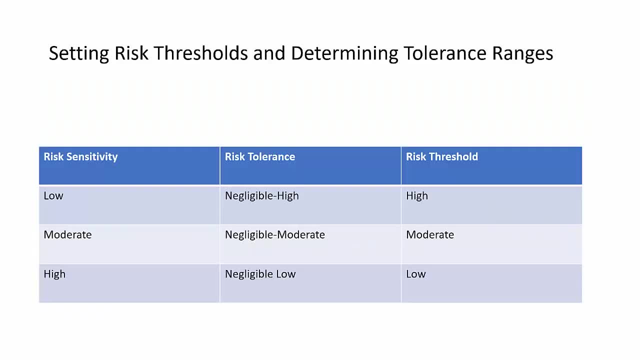 I follow for my project. okay, let me show you that. okay, so this is a formula which I used when I am basically setting a rise tolerance. so here you can see: risk sensitivity low. in that case, risk tolerance is basically negligible. high and risk threshold is basically high. what is the meaning? see if I am running. 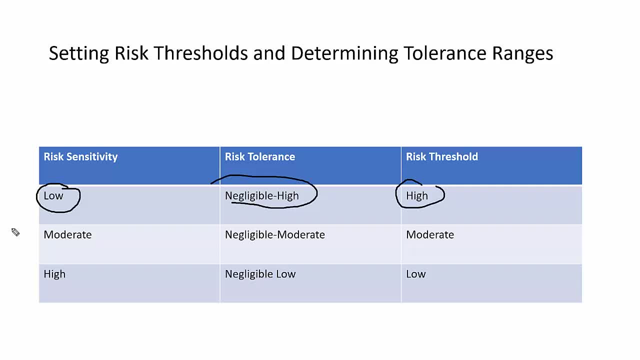 a startup example. okay, I don't have anything to lose. I mean, I'm in a business where I want to to earn customers, i want to build competitions, i want to buy more business. so in that case i will take more risk. so in that case my risk tolerance will be high because i don't have anything to lose. 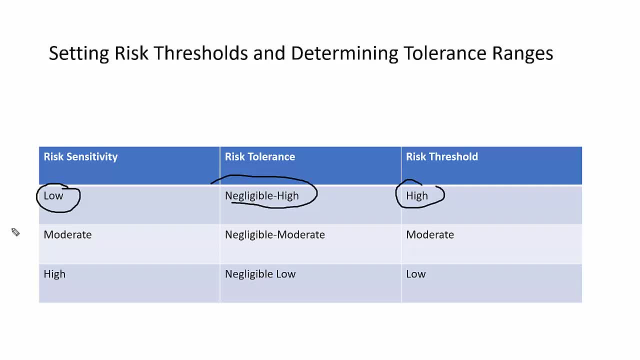 but company like big four or another banking things and all that, recently svb and all that, even they basically take a minor decision, they have a big impact. so in that case, for in that their perspective, their risk tolerance are basically low because they know very well if 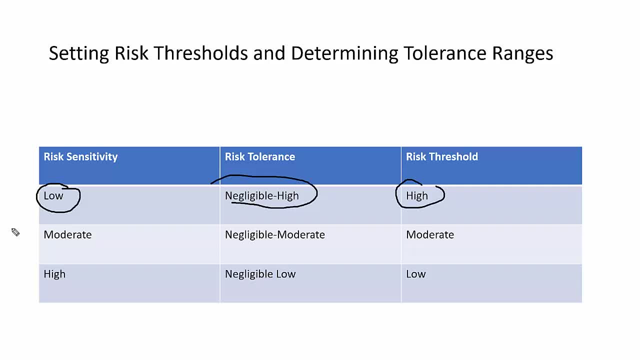 they go for any risk, for any activity, they'll have a big impact. so think of a risk threshold as a highest level of acceptable risk exposure for the resources. so, if you remember, we stated that risk threshold is always inversely proportional to the risk sensitivity level. so if you have a high sensitivity to risk- i repeat, if you have a high sensitivity to risk- 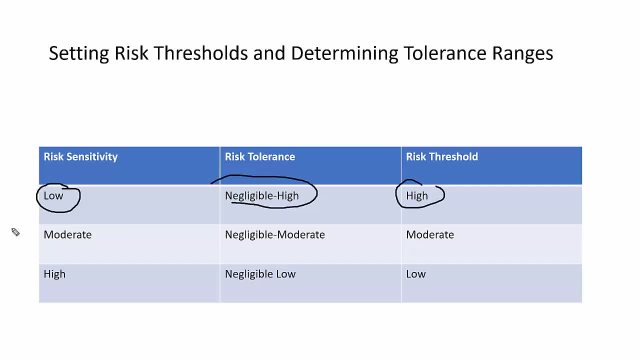 then you should have a low threshold for the risk, okay, so resource with the low sensitivity to risk is a high sensitivity to risk. so if you have a high sensitivity to risk will have a higher threshold for the risk exposure. so risk threshold is the upper bound for the risk. 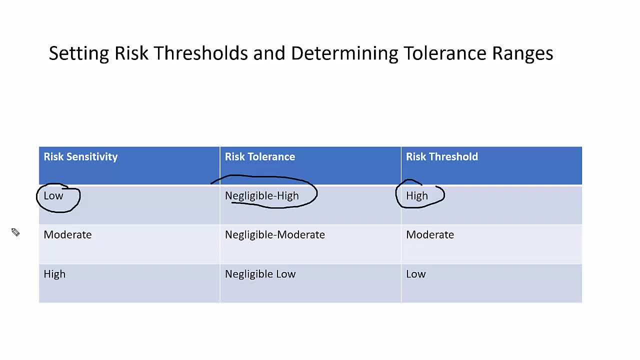 tolerable range and risk tolerance range define the lowest and highest level of acceptable risk for the resources. okay, that's the most important thing. so if you have a high sensitive to high sensitivity to risk, then you should have a lower threshold and resource with a low sensitivity of. 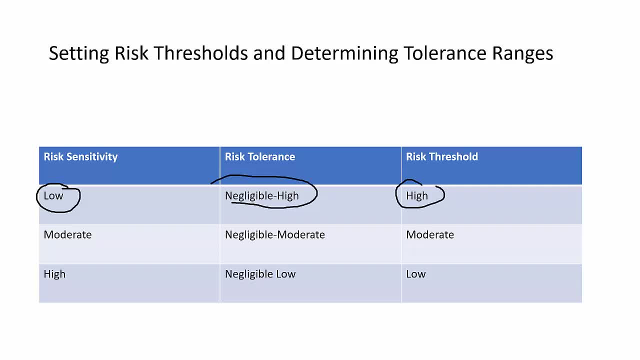 the risk or low sensitive risk. then we have a, you know, high threshold. so risk tolerance is basically driven by that factor only. so here we can see: risk sensitivity is basically low, risk tolerance negligible. no, we have a high. okay, we can take high risk tolerance, because the data 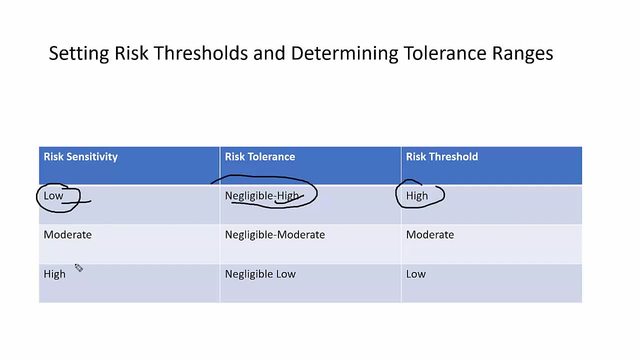 is no, and risk threshold we have set is high. but in the case of high risk, sensitivity in that tolerance will be low, so risk threshold is also low. how? let me give you an example. this is basically my server. okay, that server is basically support this business process, this business process, every. 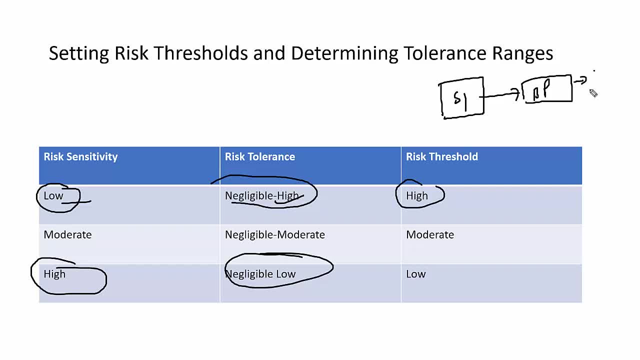 second, generating a good amount of dollars for me. for me, in this case, the risk sensitivity is basically high, so in that case my risk tolerance is basically low. so anything happen, even for a second, i cannot bear it. so i will understand the business management requirement. i understand. 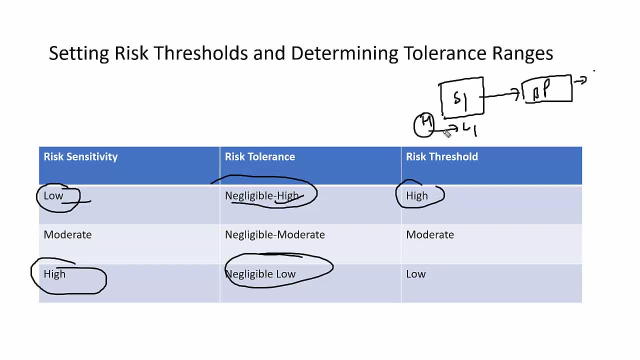 cinema requirement to understand how critical is the business process. so according to that, i will set the thing. so in this case, if any attack happen like there is a virus and virus is a threat, it is a risk, and if server is basically down even for a one minute, the impact is basically high. 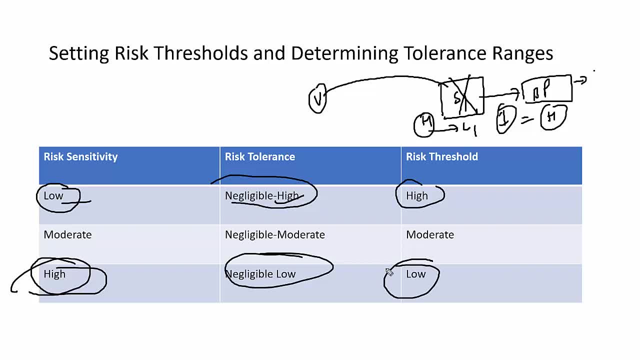 because risk sensitivity high and threshold is basically very low for them. so, according to that, we need to prepare the things, we need to mitigate the risk. so that is how, based on the tolerance and based on the beyond, the appetite will take action. so once you have all these things, then you 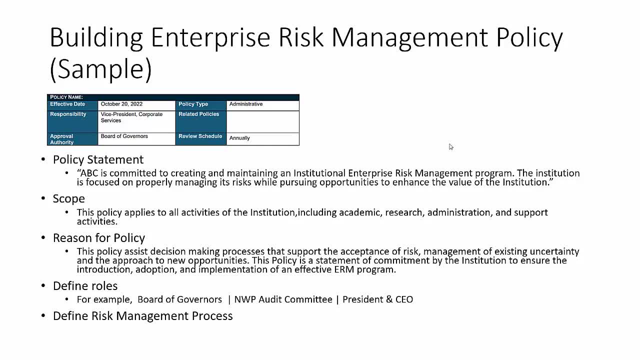 formulate and create a policy. see, policy is the first thing you create, okay, in which you define the policy statement: risk management is applicable for which particular area. okay, what is the reason of policy? define the role and then we define the risk management process. so all these things is basically part of 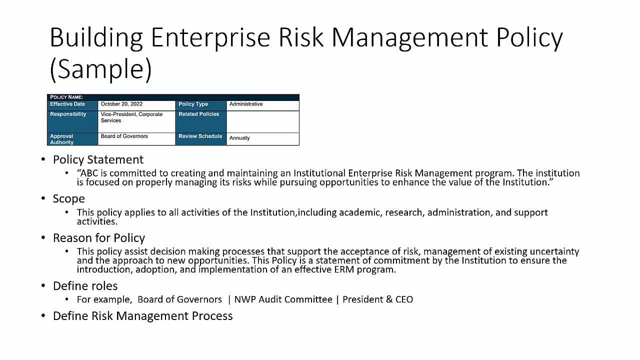 the policy. you know, when i started a session, i already shown you how the policy look like. okay, so your strategy, further to that, include the policy. okay, so first we create a strategy, then we create a policy. okay, because policy set the expectation, policy is a, you can say, governance. 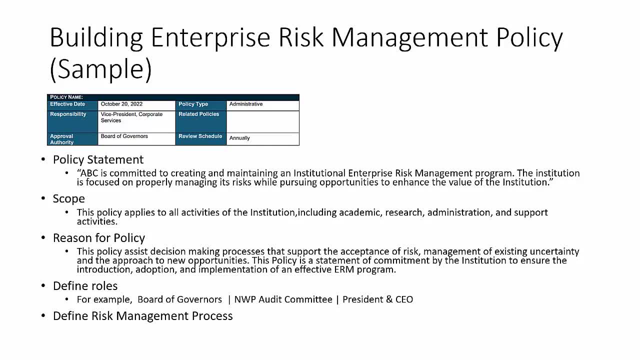 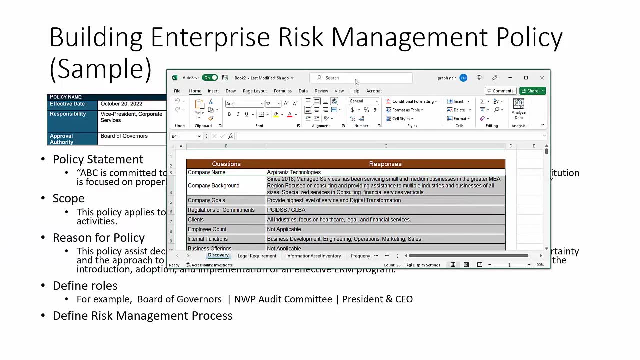 it's a foundation for a risk management governance- okay, and policy is a part of a strategy. now we are moving on the operation level, where we are conducting a risk assessment. now let me show you the excel sheet. so this is the sample excel sheet which i have created, okay, for my organization. so here you. 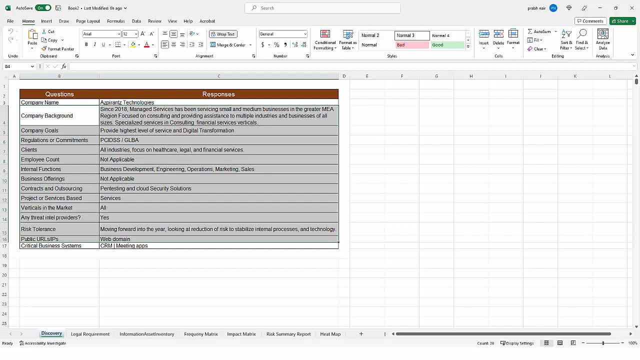 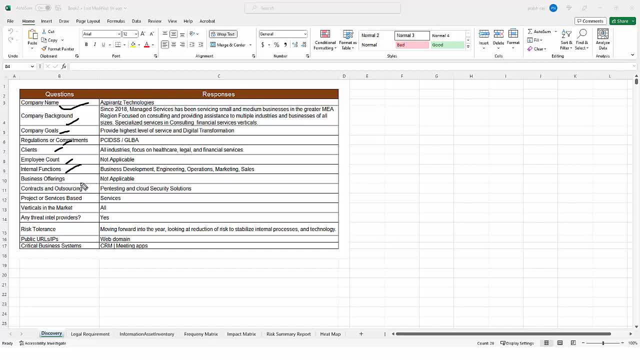 have any functions like here? we have business development, engineering. what is the business offering contracts, outsourcing, do we have? what kind of vertical in the market we are into? all okay, any threats? definitely we have. what is the risk tolerance? moving forward, 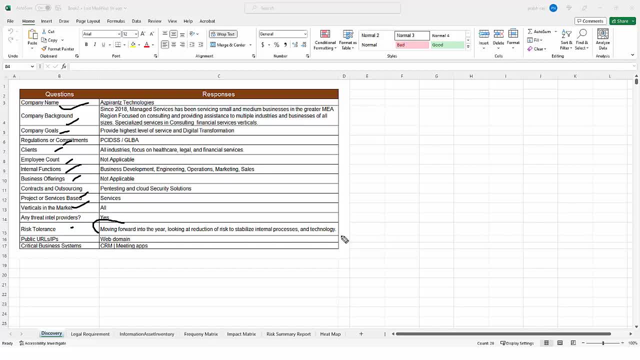 into the year, looking at reduction of risk to stabilize the internal process and technology. that is basically my risk tolerance. what are the public IPs we have web domain. what is the critical business system? CRM meeting app. so this is something is my first step. 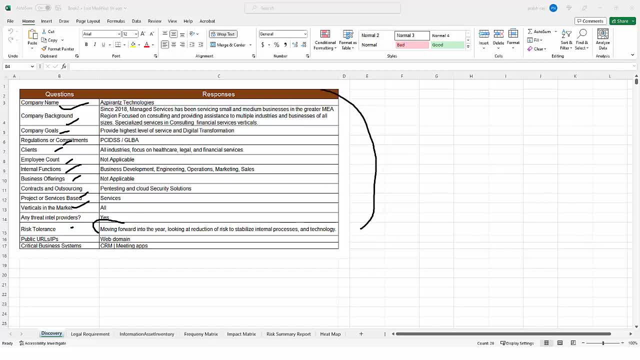 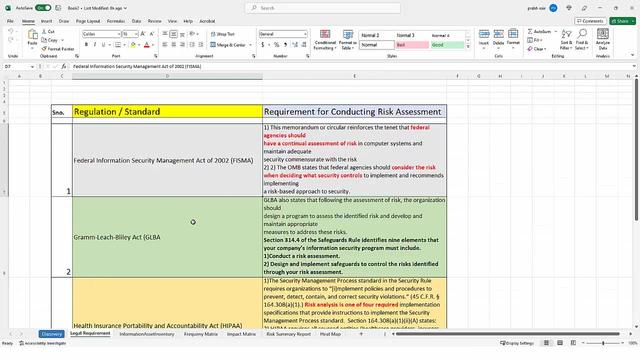 which is basically called as a discovery, where I want to discover the information about the organization. then, on the next step, I will document the legal regulatory requirement. you know, suppose, infosec, you know Aspen and technology. they are basically doing a business in US, they are doing a business in UK. so when they are working in these respective 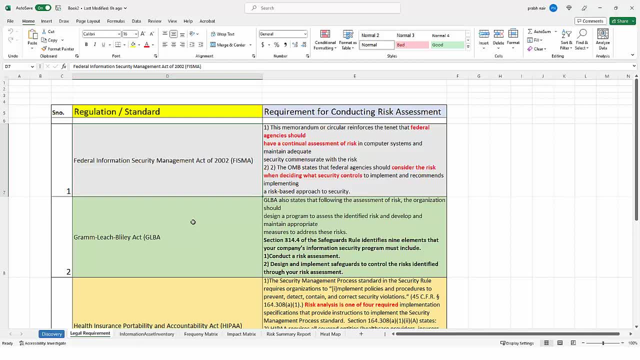 countries. okay, they have to abide with legal regulatory requirements. so in this case, I have to see, okay, how my company is going to be impacted by the regulation. so, example, like I am operating my services in US. example, okay, so I need to be comply with FISMA. okay, I need to be. 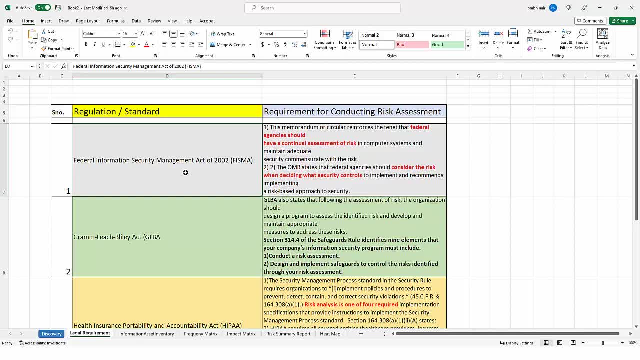 comply with the FISMA and FISMA also have a requirement that you must do risk assessment. so I am not doing a risk assessment to check what is the level of compliance we need to follow, but as a company it is mandatory for me to have a regulatory requirement have. 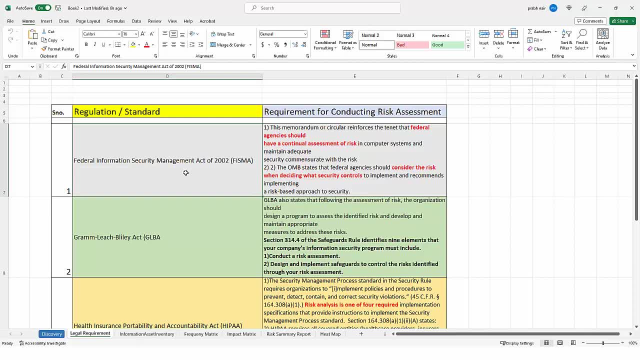 a risk assessment requirement in the organization. so FISMA say you need to do risk assessment. you can see it is clearly mentioned here this memorandum or circular. it infose the tenant that federal agency should have a continuous assessment of risk. so it is a regulatory. 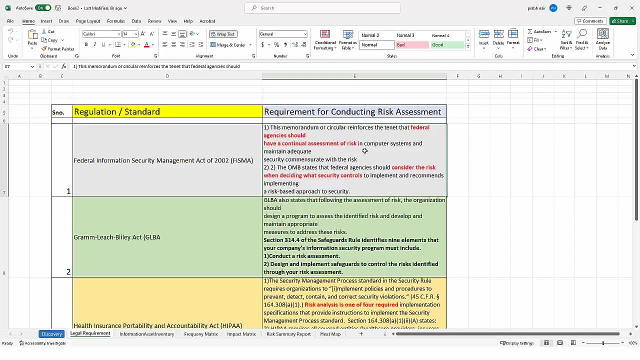 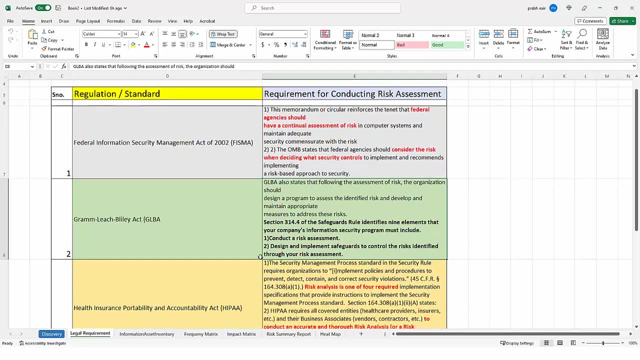 requirement. you must do risk assessment in the organization. now, as I said, I want to comply with GLBA. GLBA also state conduct the risk assessment according to section 314.4,. then if I am operating my services more in the health care I need to comply with HIPAA. 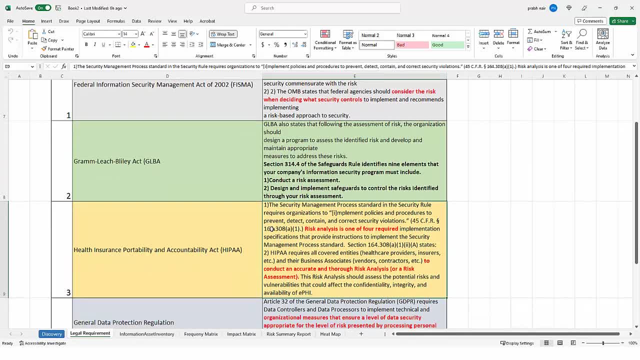 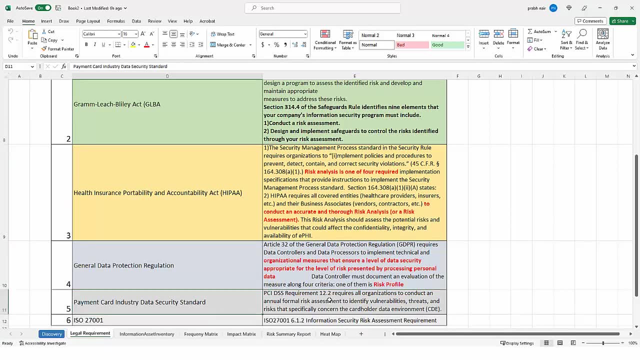 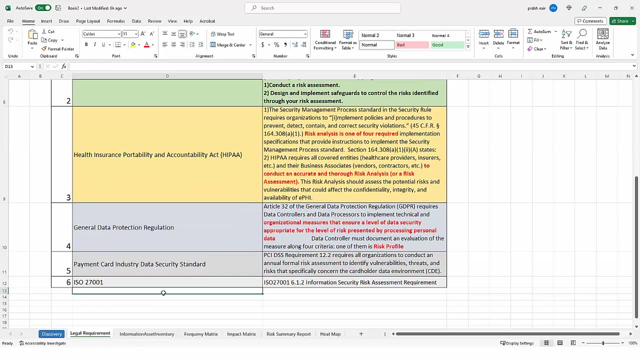 HIPAA has their own requirement of conducting a risk assessment. okay, then, if I go for GDPR, they have article 32. talk about You need to measure the security controls. PCSS has a 12.2 requirement, you need to have an annual formal risk assessment and ISO 27001 itself basically saying that you need to have. 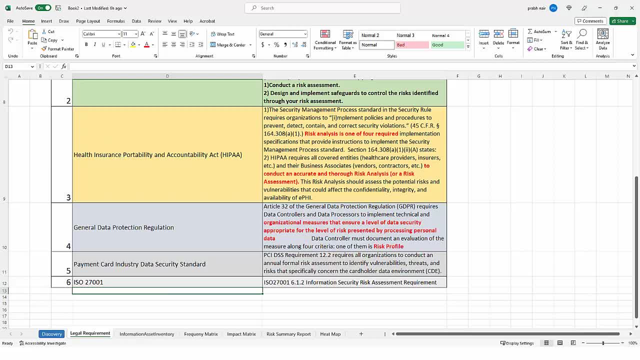 a requirement of 6.1.2, which is called information security risk assessment. so this is also risk assessment is. sometimes it is not about the business requirement, but it basically come from a legal and regulatory requirement. okay, that is the most important thing. 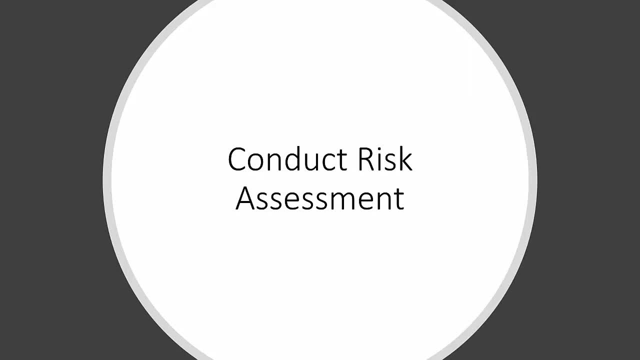 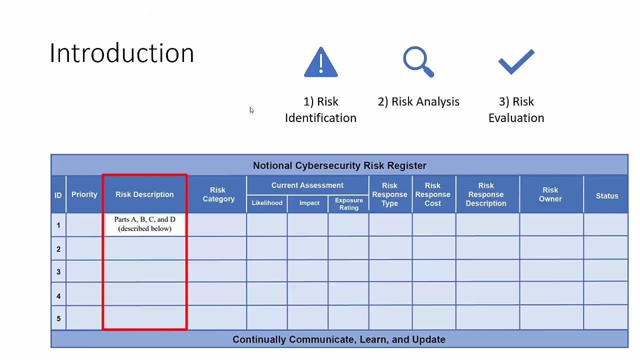 So once you basically create a policy strategy, now we have to start our action. how to conduct risk assessment? okay, So when you're doing a risk assessment, risk assessment basically have a three steps: one is identification of the risk, second is analysis of the risk and third is called as a risk. 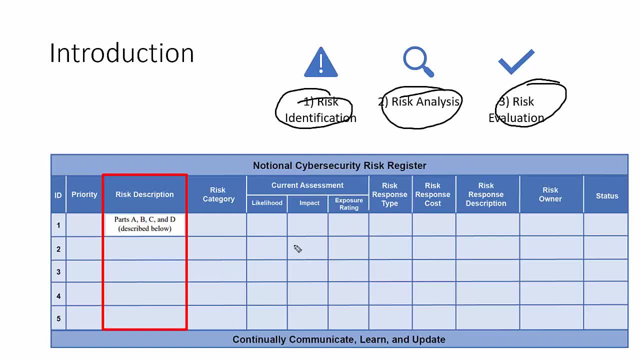 evaluation. okay, So this is just an example you know, mentioned in this PPT. you know the risk ID, the priority description category, what is the likelihood impact exposure rating control type. so we're going to discuss each and every step in detail. 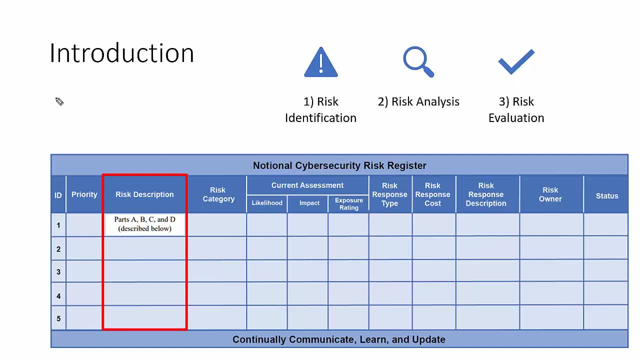 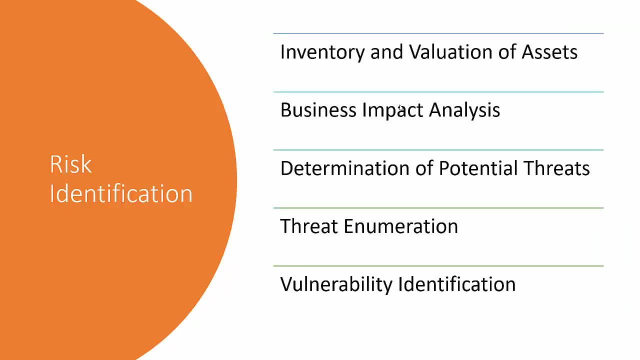 So we're going to start with the first part, which is called as a risk identification. so when we're talking about risk identification- risk identification- the first step is we need to know the value of assets, we need to know the inventory of assets, because when you're 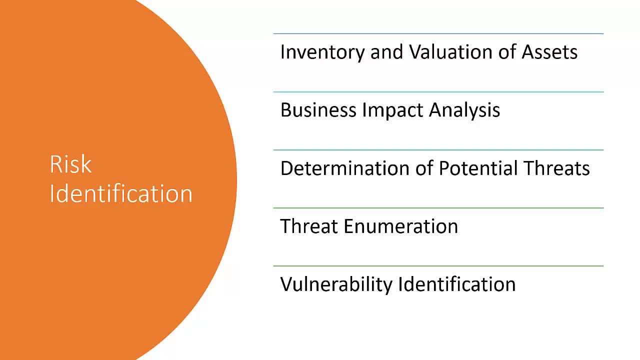 doing a risk assessment underliners. you don't know what. you know what asset we have against what you're doing, going to do risk assessment. So for risk assessment, the first thing we need to understand the inventory and valuation of asset. okay, So I want to show you my Excel sheet. 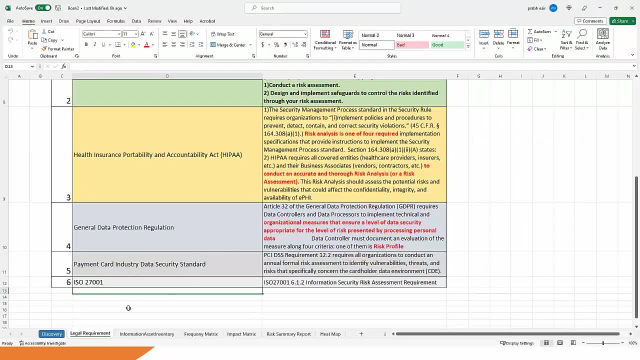 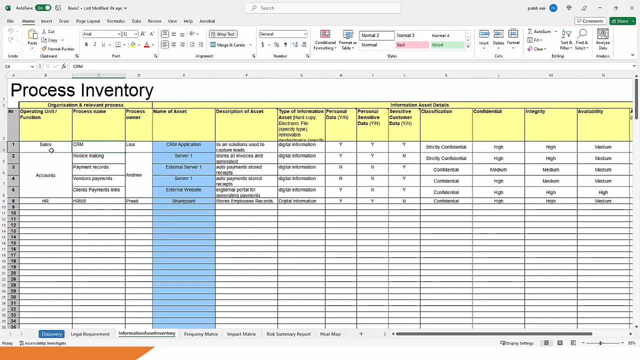 Okay, In which you get the information about the inventories. so here you can see I have a CRM process and the affected unit is sales. the process owner is Lisa. the name of the asset is CRM application. okay, The description of asset has been given. like it is a solution capture leads. the type of 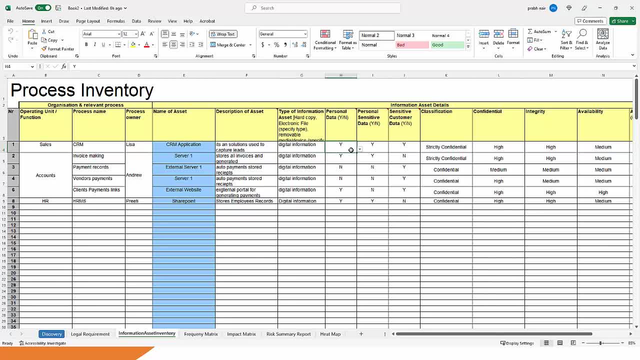 information we're capturing is digital. does it capturing personal data? yes, we capturing email ID. does it having a personal sensitive data? yes, because we sometimes capturing address. are we capturing sensitive customer data? yes, So according to the company's classification process, it is strictly confidential okay. 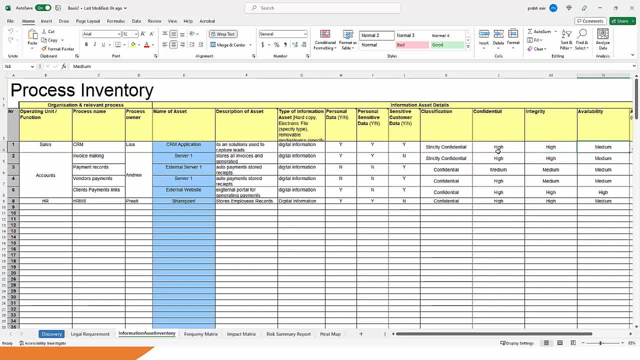 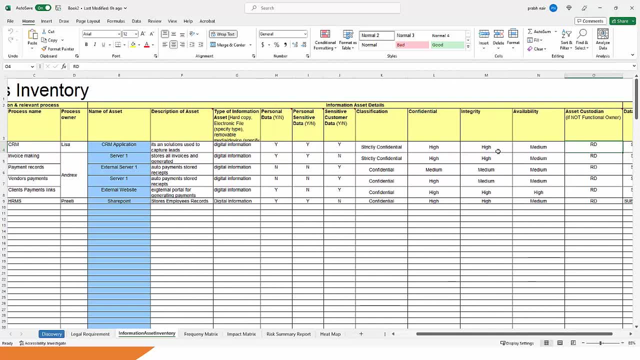 Confidential level. impact is basically high. integrity. high availability is basically medium, because for us, we need to protect this information from disclosure. we also give the information about who is the custodian, like in our team. we have RD and detention period is subject to the business requirement. okay. 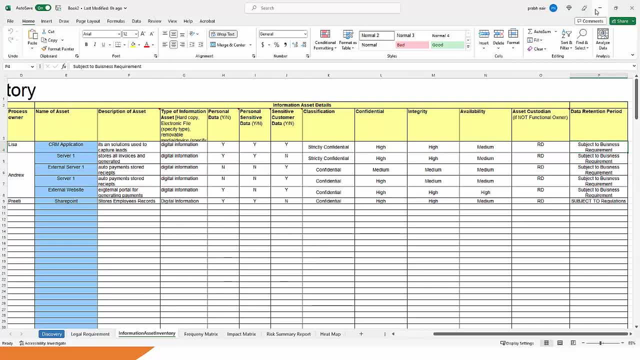 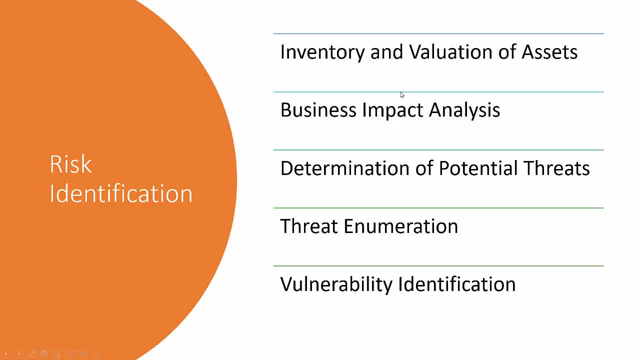 So this is how we have maintained the inventory of assets. Now, here you can see. once you have an inventory of assets, we identify the value of assets. value is two type: qualitative and quantitative. okay, Then it is not possible for us to give attention to all the assets. so, based on the value, we 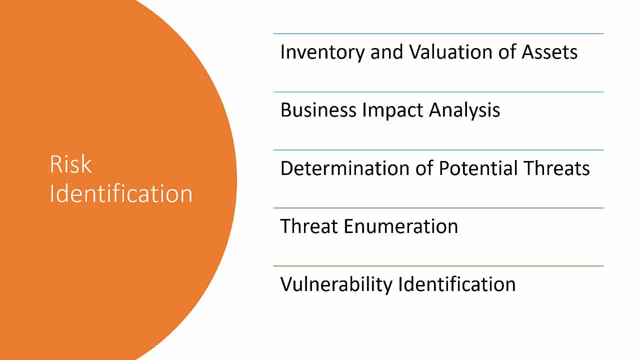 drive the BIA. BIA is all about what is important, what is not important. so that is called as a business impact analysis, Because if you have a 5000 assets and you want to do risk assessment of 5000 assets, 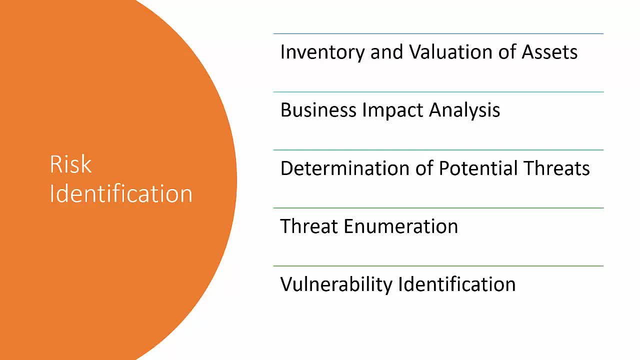 it is not possible on the same time. you can do that. So we do the BIA to identify from 5000 which process is basically important, which process is basically critical. okay, Because it is not possible in one go, I can do risk assessment against the 5000 applications. 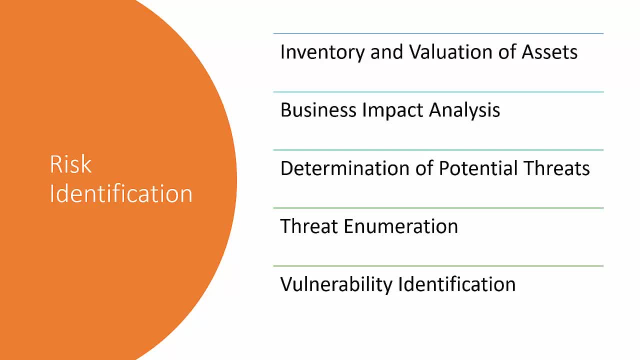 So we do the BIA to identify which one is critical, which one is not. So with that BIA, I am going to pen down all the potential threats. okay, I need to pen down all the potential threats, I need to extract all the threats and then 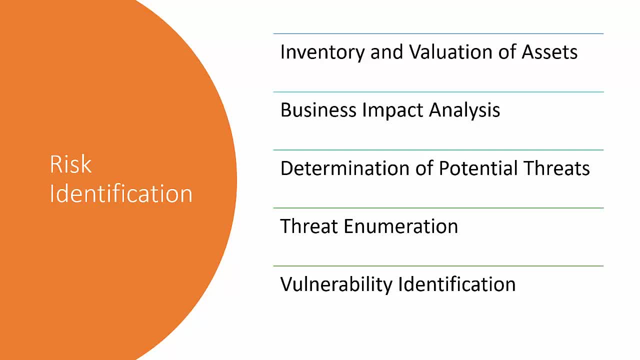 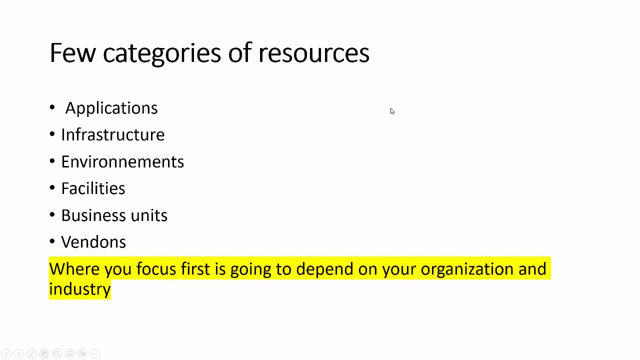 I need to identify the vulnerabilities which is associated with the assets. Okay, So I need to pen down. I need to obtain the list of vulnerability data. okay, So question is how to further categorize the assets. So here we have a few category of assets or resources, like application is there? okay, 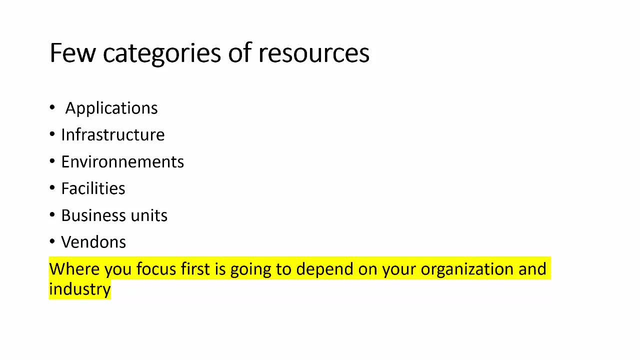 infrastructure is there okay. environment is there. facility is there. business unit is there. vendors is there okay. So when you focus first is going to be depend on your organization industry. So when you focus first is going to depend on your organization industry when you focus. 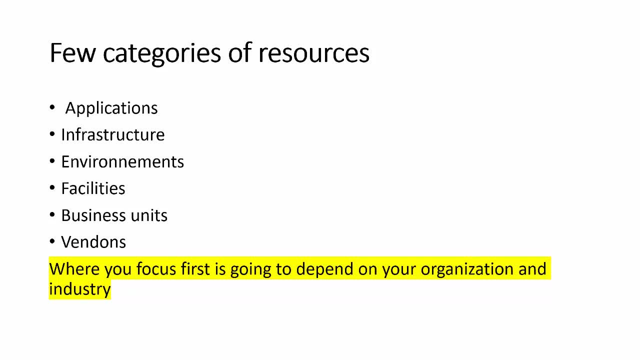 first is going to depend upon your regulations. So example like: if you are an internet service provider, you might start by profiling your infrastructure okay, such as network devices, DNS server and so on, But if you are an application service provider, you would like to start with the application. 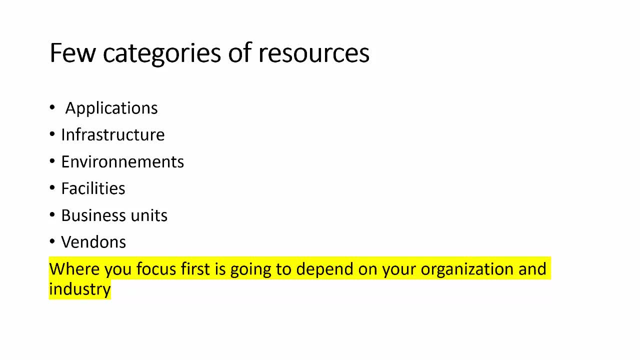 that you host. Similarly, the organization that make heavy use of offshore developers might focus on their vendor profiling first. So understand the business you are in will help to guide your priorities. You don't need to address all this area Right. Get out on the gate, pick your battles accordingly. 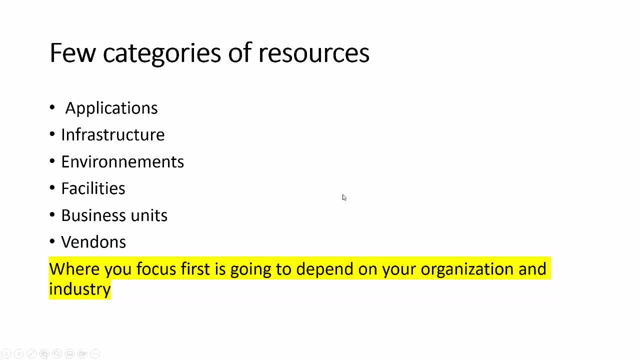 Okay, so that's the most important thing. So when you focus first going to depend upon your organization industry, that's the most important thing we have. Sorry for the correction, it is vendor okay. So here we have example. like we have to capture the details in this order, like resource owner. 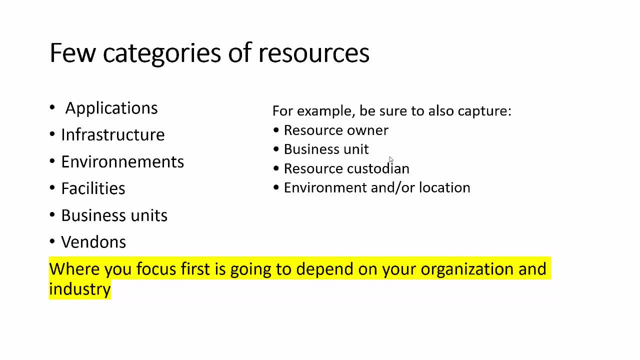 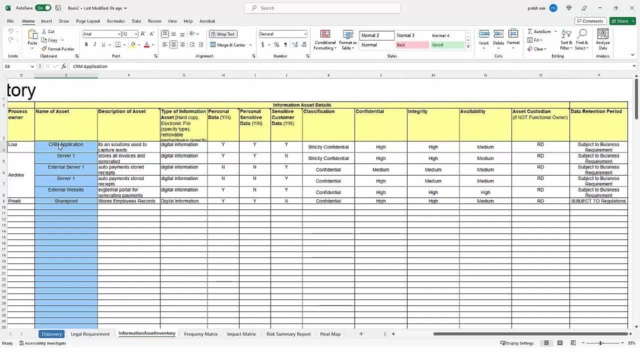 okay, business units, resource custodian, environment. I've used the same thing, but more in detail. I mentioned the asset custodian, I mentioned the type of information I'm capturing and what is the name of assets. So this is a sample. 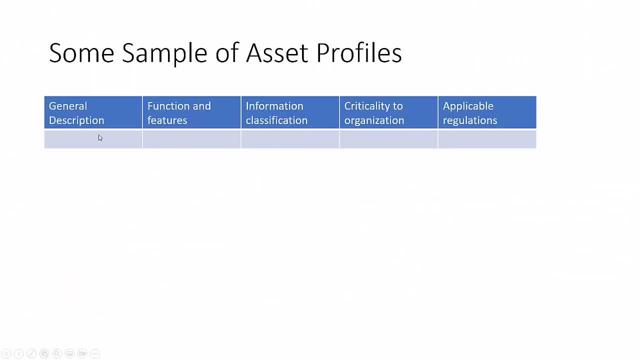 Asset profile we have. we create, okay, general description of asset, okay, function and feature what the asset is basically offer. what is the classification of information, what is the criticality and that information does it applicable in any regulations. 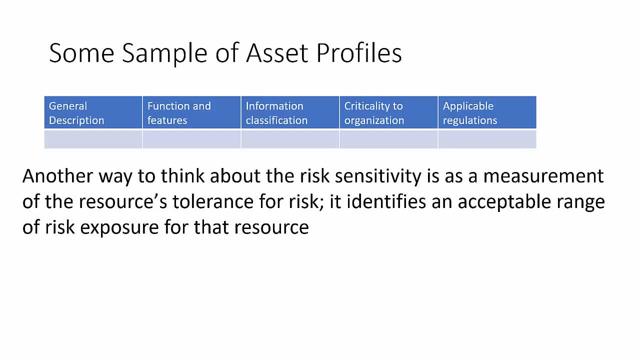 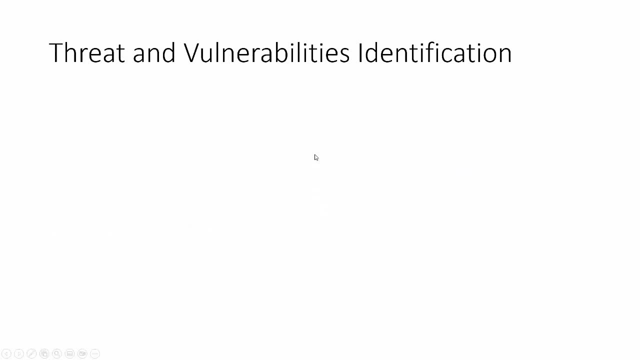 So, as I said, another way to think about risk sensitivity is a measurement of the resource tolerance for risk and it identify an acceptable range of risk exposure for that resources, because risk exposure we have to identify in the asset profile. Okay. Now, once you basically have assets in detail, okay, then we need to identify the threats. 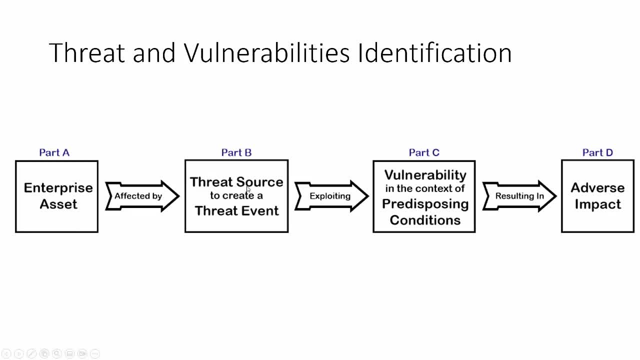 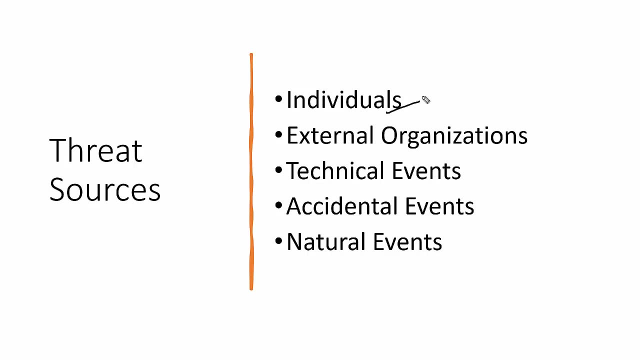 and vulnerabilities which we already discussed. they're going to enterprise effect by the threat source which exploiting a vulnerability and that result into the adverse impact. So question is how to identify the threat source. So we have a different type of threat source example, like we have individuals threat source. 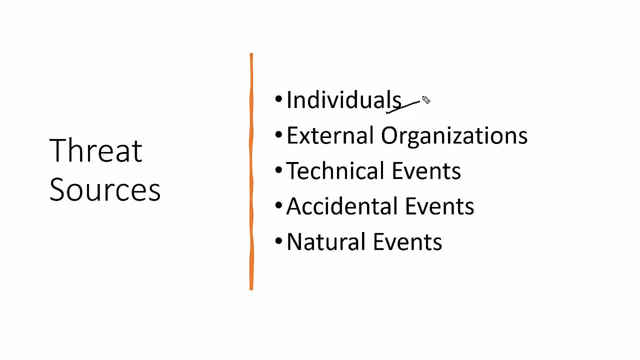 example like employee, contractor, customer, client service provider- okay, hackers. these are examples of individuals. Then we have external organizations like activists, criminal individuals, terrorist and all that. Then we have some technical event which can be a threat for us. you know, organized crimes. 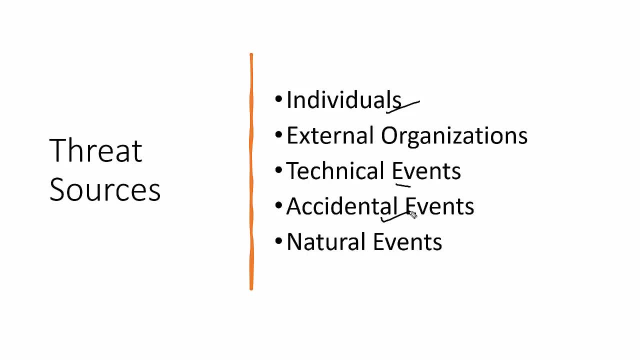 and all that. Then we have accidental crime, where the employee click on some links and all that okay. Then we have a natural events like floods and everything. So it is very important to pen down the possible threats. My suggestion is that first identify the vulnerabilities. 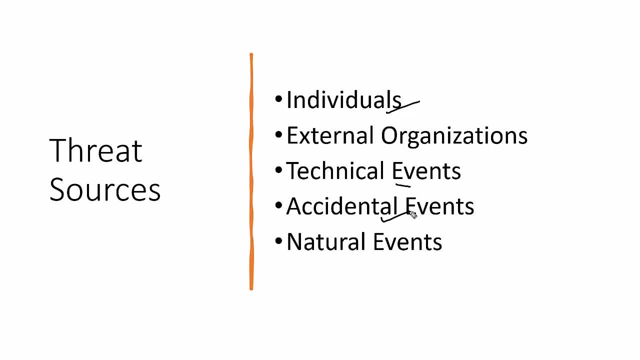 And then identify what are the threats against the vulnerability exactly. that's the most important thing. So let's take example: we have a server- server is basically connected on the internet, So and we have discovered server 23 port is open, So that is also a functional port. 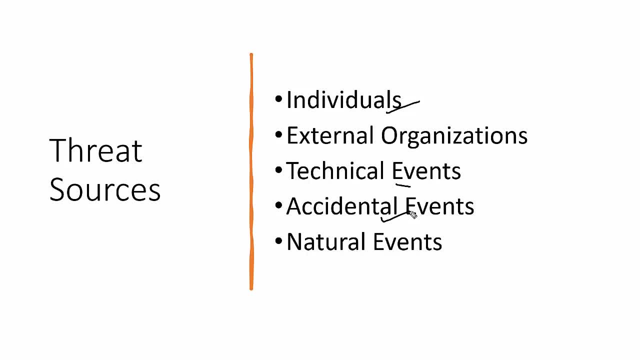 But also there is a weakness that, okay, anyone from that particular port can able to connect with the server. Okay, so if there is no threat against that vulnerability, there's no need to patch that. So it's your call. You can just pen down the possible threats or first identify the vulnerabilities, and 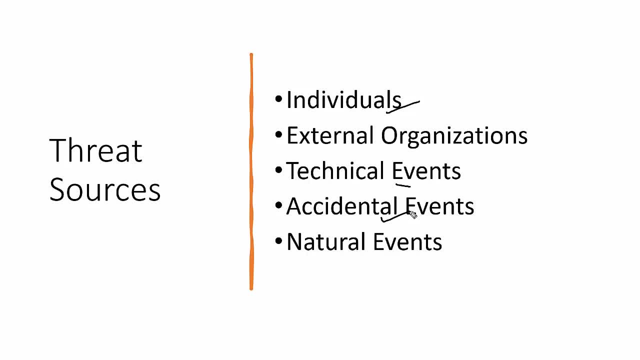 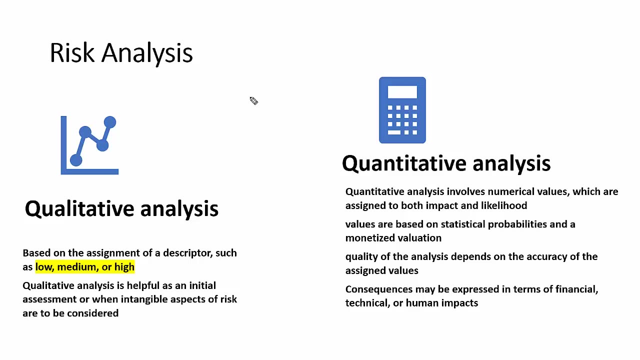 then identify the threats. So all these things we have to do in the identification stage. So this is all the activity. So next we move to the next part, which is called as a risk analysis. Okay, Okay. so next thing is basically we have a qualitative and quantitative risk analysis. 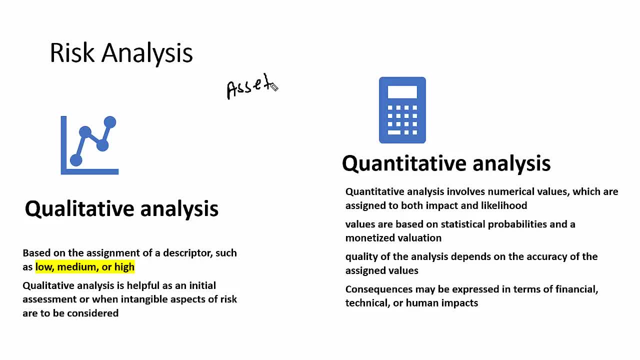 See, we identify asset, We identify threats And we also identify vulnerability. And now we are in a position that, okay, if the threat is going to exploit the vulnerability, what is the impact on the asset Impact mean? what is the overall impact? 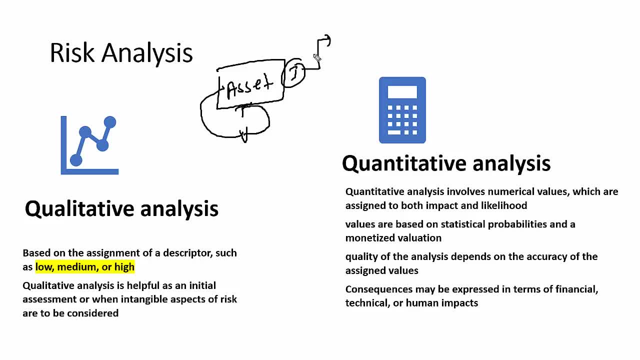 What is the level of impact That we need to calculate? We know there is a hacker is going to hack the server and by which he can able to gain access to the data, But if he able to access to that data, okay. what will be the impact on the organization? 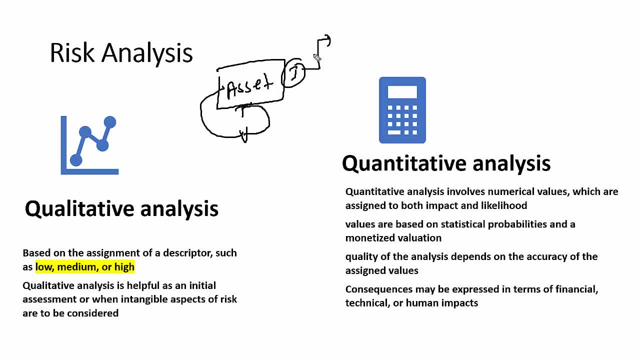 Like you know, the organization is answerable to regulatory authority. Okay, There is a cost involved in that. Organizations suffer the business loss because of the disclosure of a data. It impact the reputation. So all these analysis we need to perform. 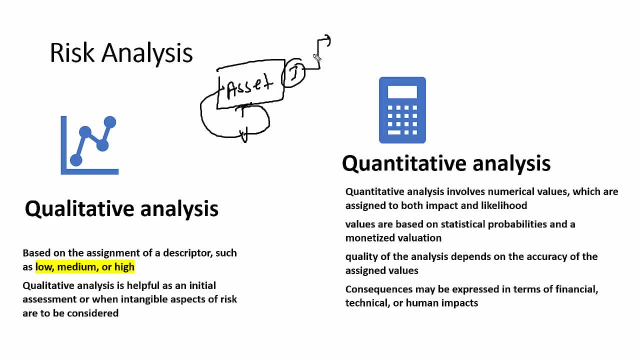 So we have a two way to analyze this impact. One is called as a qualitative analysis, where we just rank the risk into high, low and medium, And the second one is basically called as a quantitative analysis, where we are using a numerical value. Okay, 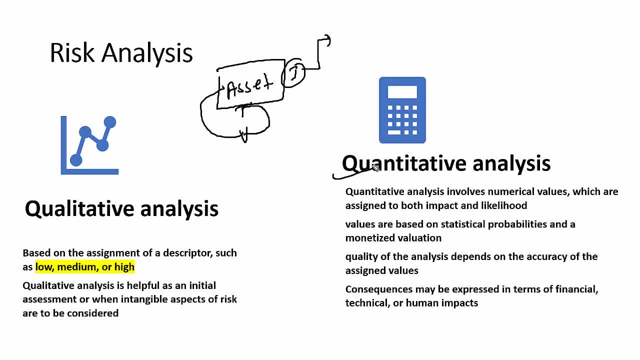 So this is something you need to understand. If you have a limited time and you need to go for a, you know, high level assessment and all that, then we can go for a qualitative analysis, But where the numbers are involved, okay. 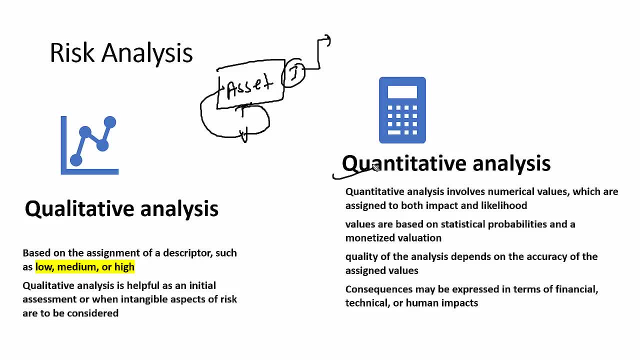 Calculations are there. It takes time, but it is a more accurate. that is called as a quantitative analysis. So qualitative is high level, fast. Quantitative is basically slow, Definitely, qualitative is basically more like a hypothetical scenario kind of a thing. 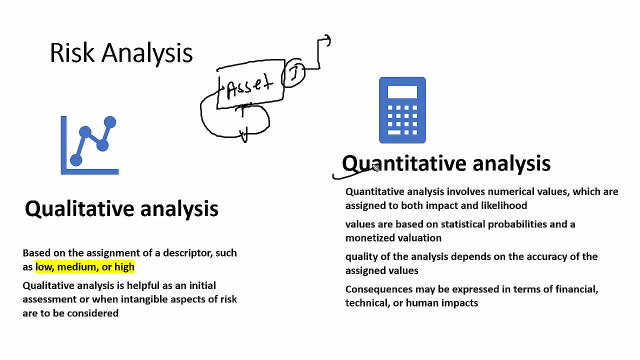 There is, a quantitative is most accurate. So when you have a historical data, it is easy for us to perform the quantitative analysis, And when we don't have a historical data, we just need to do the higher high level analysis. We go for the qualitative analysis. 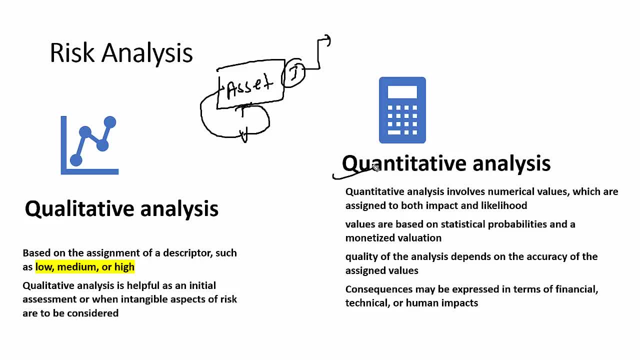 I have seen some organizations where they start with the quantitative and then they go with the qualitative. I have seen that such kind of an organization also. So I'm going to explain the practical of the quantitative, but first the qualitative. first we discuss about the quantitative analysis from the theory. 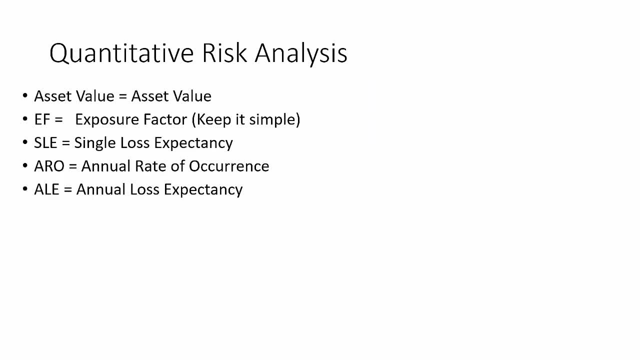 Okay, Theoretical perspective. So in the quantitative we basically follow this formula: asset value, exposure factor, SLE, ARO, ALE. okay, So these are the parameters we have that we used in using for a quantitative risk analysis. 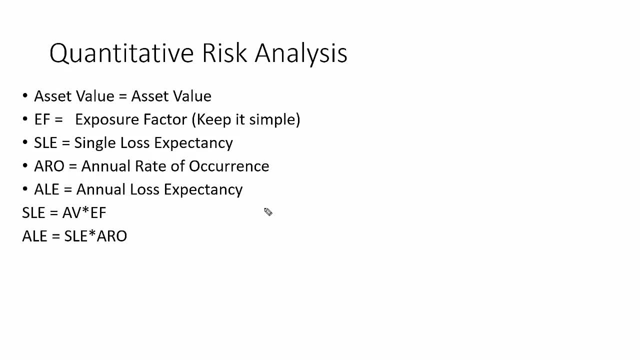 So in the quantitative risk analysis, the first thing we need to use the SLE. SLE basically stand for single loss expectancy, and how we calculate with the help of asset value and exposure factor. Exposure factor is called as a percentage of the asset loss. 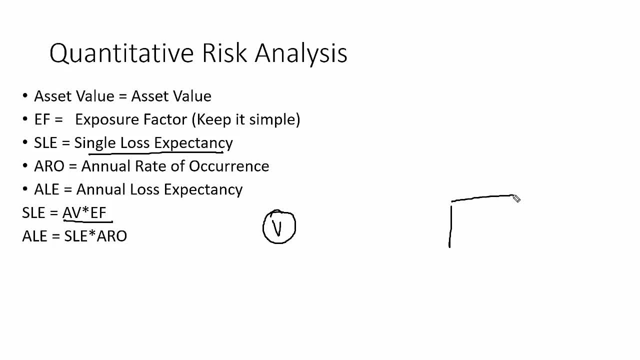 Example: there is a virus and there is a server. okay, Now server basically having an asset value is suppose $10,000.. If virus basically attack on the server one time, if one time virus attack on the server, okay, Server will be down. 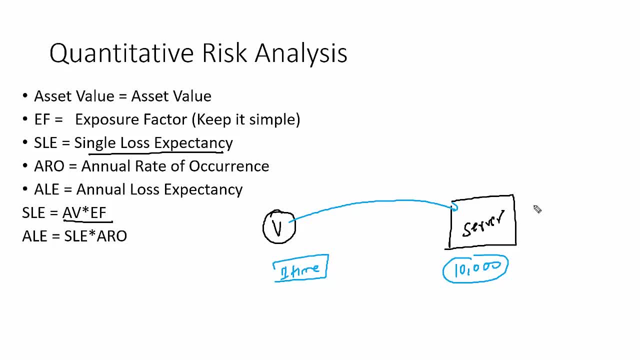 Okay, But the question is, if server is basically down, what is the impact that we need to calculate? So formula is basically: SLE into asset value, into exposure factor. So here the asset value is $10,000.. I'm assuming if server is down, it will. it will basically down for everything. 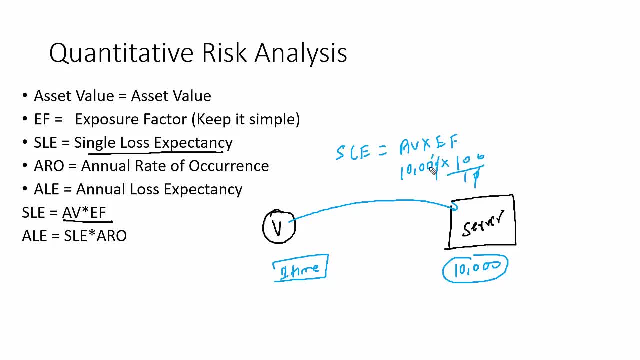 We keeping a hundred percent. Let's take example: Okay, So it will be coming around. overall SLE loss for me is $10,000.. See So when we work in the production we always take exposure factor as a hundred percent only, because we cannot assume. 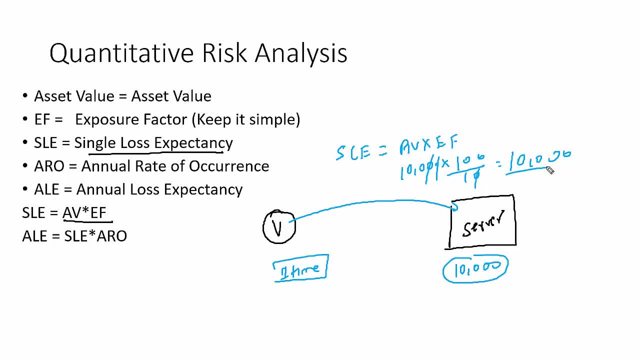 So exposure factor is all about percentage of loss. Now we assuming that, okay, if one time server is down, even for one hour, the asset value reduced to $8,000.. Okay, So formula then will be: SLE Asset value is $10,000.. 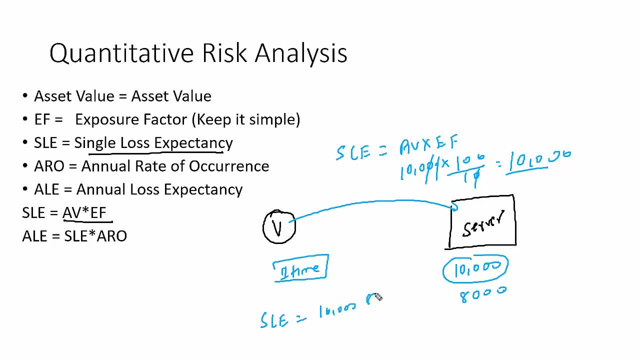 Okay, Exposure factor of 8,000 of 10 is 80%, because we've always given a percentage, So it will be coming around. SLE is $8,000.. So single loss cost me $8,000.. Now, based on the single loss expectancy- $8,000, I'm going. I'm not going to invest the antivirus. 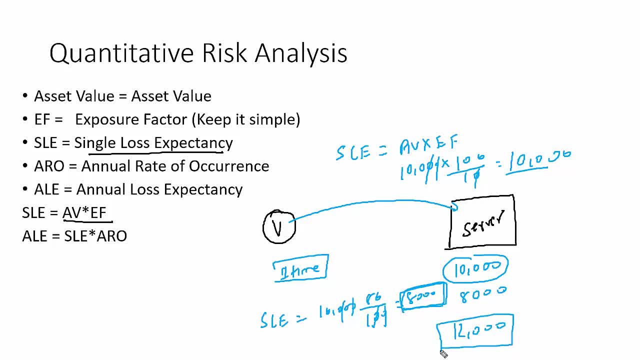 because antivirus coming around cost is $12,000.. So I'm not going to invest $12,000 to protect my $8,000 loss. So that is why we never take a call based on SLE. We always take a call based on a ALE. 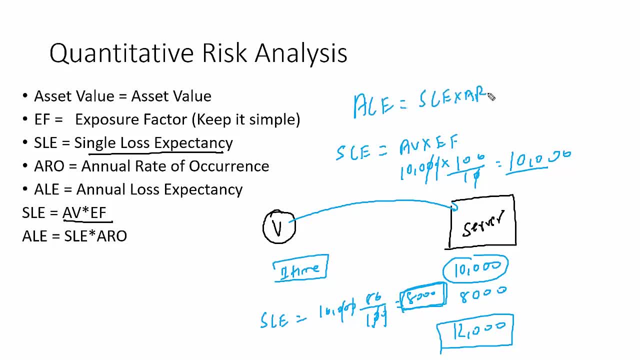 So in the ALE the formula is SLE into ARO. Okay, Okay, Okay. Now SLE basically is $8,000.. And this wire has basically attacked, suppose, six times in a year, So it will be coming around $48,000.. 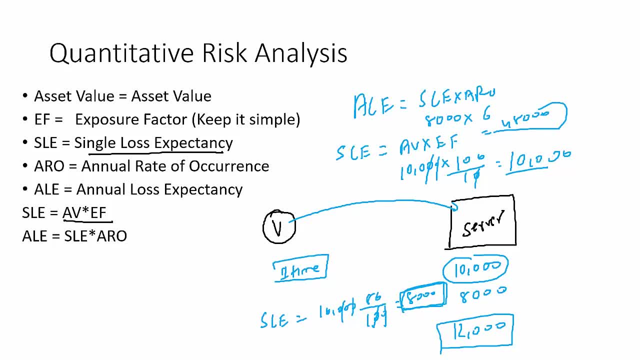 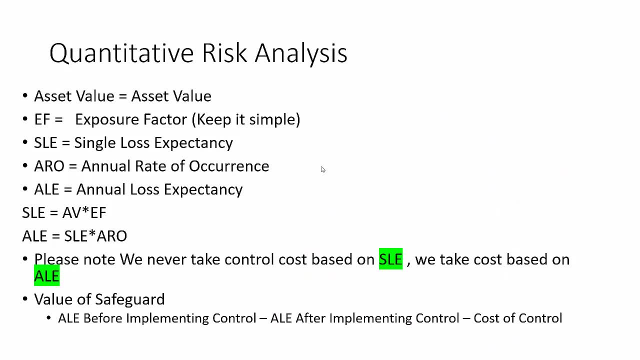 Now it makes sense to spend $12,000 to save $48,000.. Okay, But one more important thing: when we're talking about the control, okay, we need to give a justification of the value of control also. So formula for that is ALE- before implementing control. 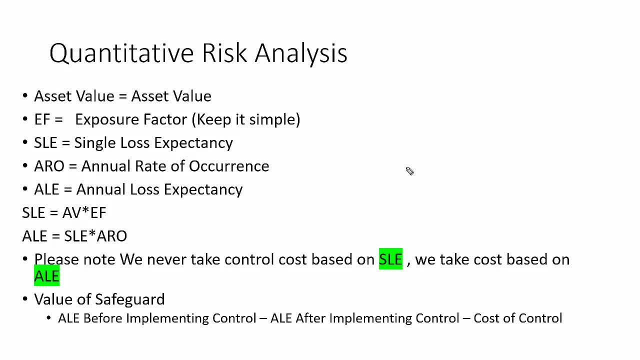 Suppose in this case the cost is coming around $48,000 minus. after installing the antivirus, it is reduced to suppose $3,000,. okay, Minus cost of antivirus is $8,000.. Whatever the value left, that is a value of the safeguard clear. 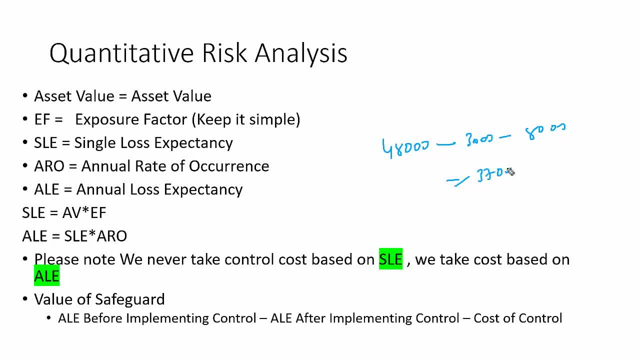 So 48 minus 840 to $37,000 is the value we have achieved from this particular control cost. Okay, So that is how you can able to measure the value of the safeguard, But that you can get only after a year. So this is basically more like a quantitative way of analyzing a risk. okay, 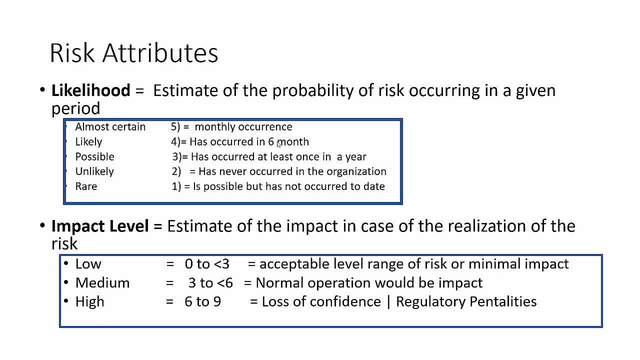 Now we have a qualitative way of analyzing a risk. So in this way we're basically using two factor: What is a likelihood and what is the impact. So when I say definition of a likelihood, likelihood is all about the estimate of the probability of risk occurring, okay, in a given period. 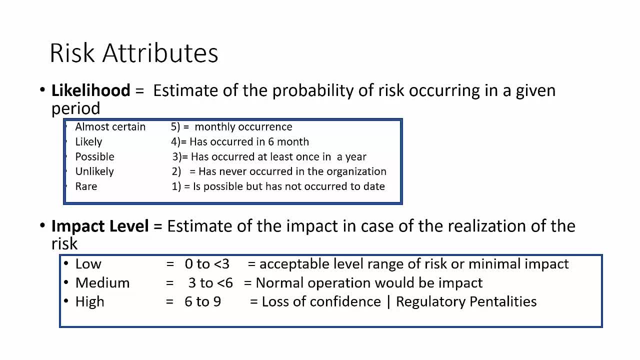 Okay. So this is basically called as a likelihood And impact. if it's happened, what is the impact? Example: like there is a server okay. Against the server, we have a monthly attacks, So threat is going to exploit the vulnerability every month. 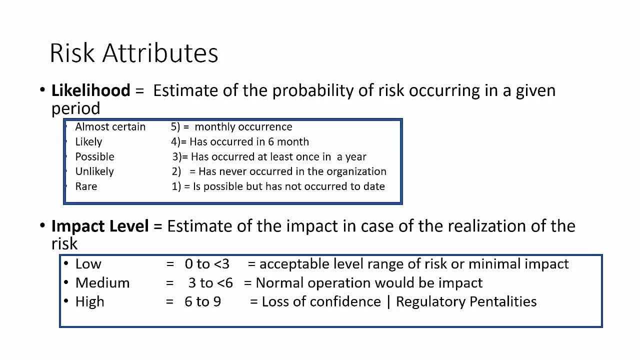 So that's the likelihood, But if it happened, the impact is $10,000,, $20,000,, $30,000, understood So? and then we map this impact with the risk tolerance and from there we get the overall. 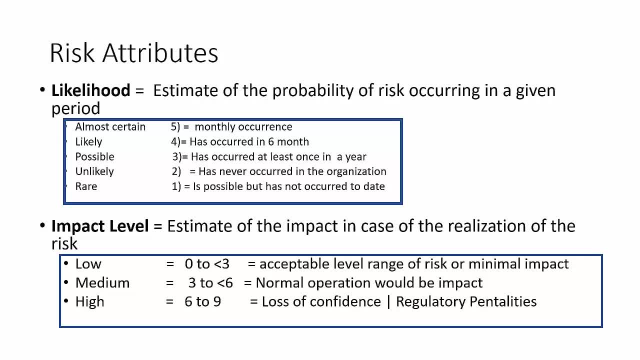 risk severity settings, Whether it is risk tolerance or risk tolerance. So the risk tolerance is high, low and medium. So here you can see almost certain like five monthly occurrence. So we give the rating. five Likely is there. we give monthly as occur in six months. 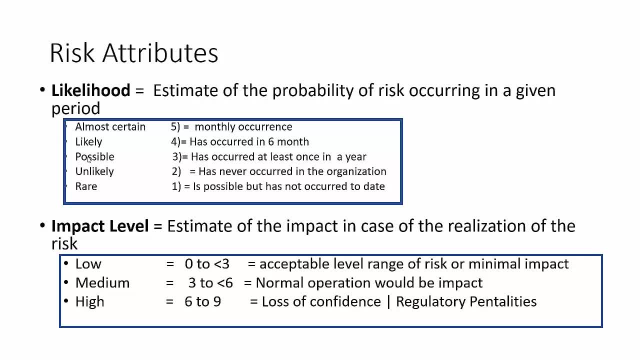 So we give the rating four. Possible is basically three. okay, Then we can see here: unlikely happened at two And rare is basically one, where the impact is all about the impact in the case of realization of risk. So here you can see, the high is basically six to nine. 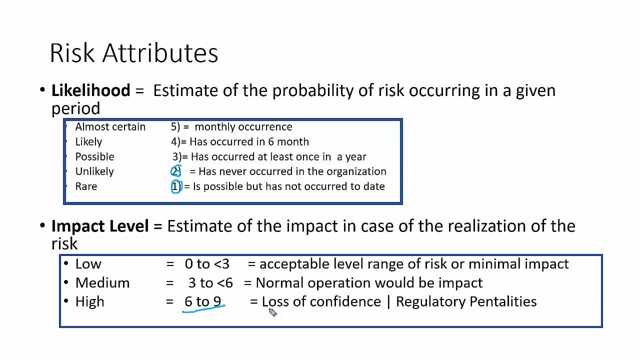 It means there is a virus. It occurs every month And the impact is basically disclosure of a data And because of that there is a loss of confidence and there is a regulatory penalty we need to pay. So impact is basically high. So we give the rating between six to nine. 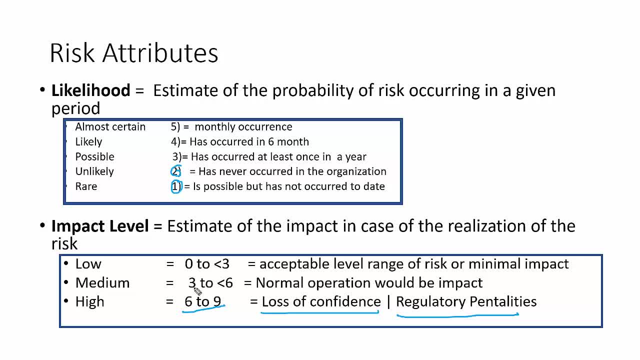 Virus attack, it impact the normal operation. So medium impact is there to three to six Acceptable level of risk within a tolerance level. we give the low. So this is how we basically measure. So I have another attribute that I'm using for the likelihood impact. 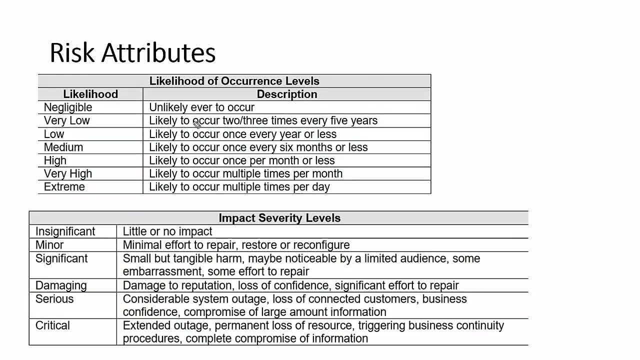 Here you can see. Now, if you can see here, this is another example. Okay, This is another example we have, If you can see, negligible, unlikely ever to occur, Very low, likely to occur two or three times every year, every five year. 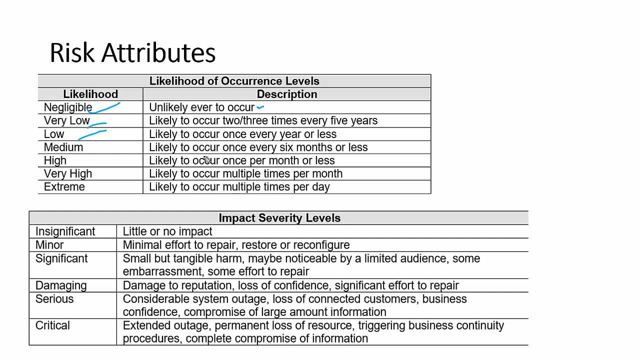 Low is basically likely to occur once every year. Medium is likely to occur once every six months or less. High is likely to occur once per month. Very high is likely to occur multiple times per month And extreme is basically likely to occur multiple times per day. 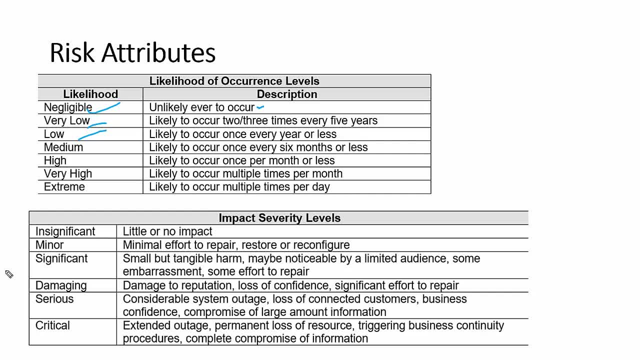 So it depends upon your risk tolerance and your nature of business, And impact is also depending upon what kind of a business you have. Like you know, you are into e-commerce, for your availability is the biggest thing. So you know, if this is attack happen, the server will be down. 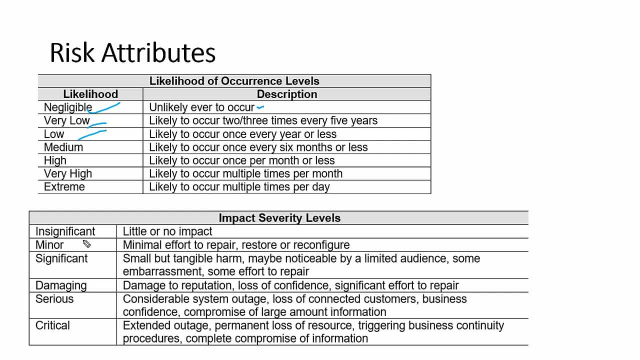 It has a big impact. So we give the rating for that impact is five. So here, insignificant, basically little, no impact. Minor mean minimal effort, significant is small but tangible. Damaging is damage to the reputation, serious and critical. 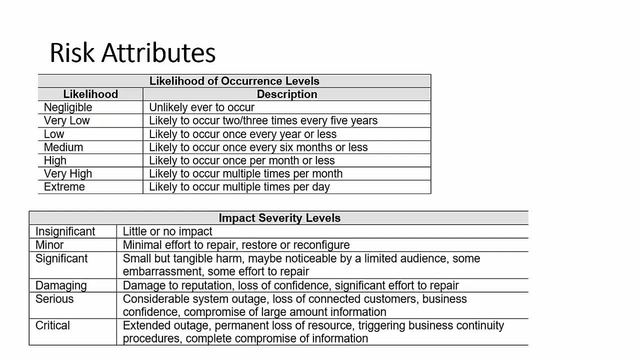 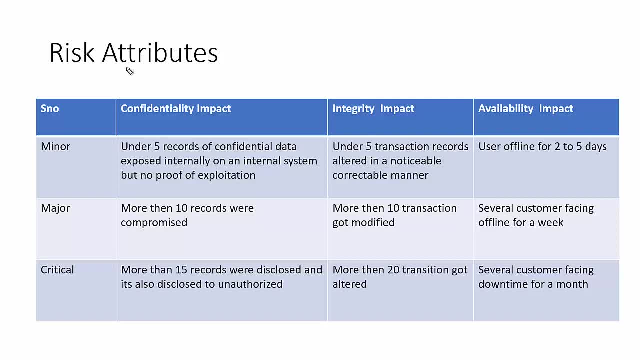 I'll give one more example So you get a better visibility. So here you can see another way we have calculated the likelihood in this one- See Sometime what happened- risk impact is mapped with CIA confidentiality, integrity, availability. Here you can see we have a server. okay, it basically store the PI data. 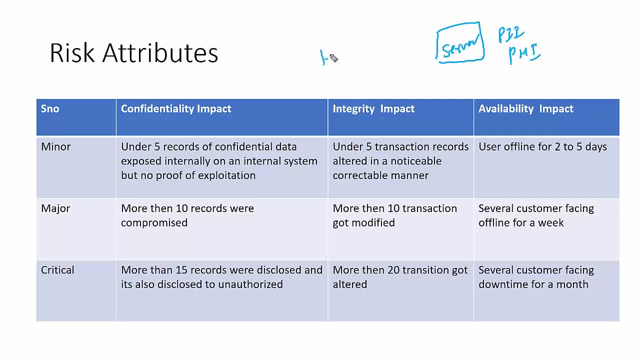 We have a server which basically store the PI data. If hacker, okay, hack into server, there's a disclosure of PI and PHI. okay, under five records of confidentiality exposed. So impact is minor but more than 15 records are disclosed. 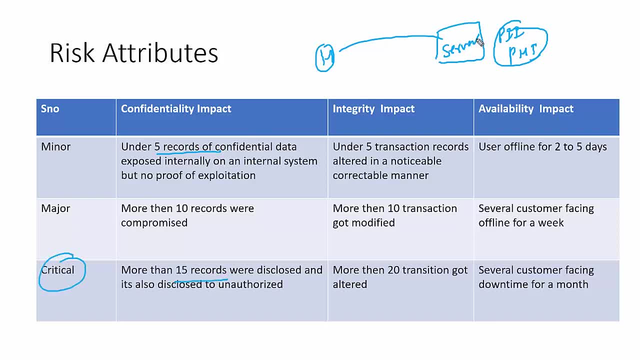 Impact is basically critical. In this case, availability is zero because there is no accessibility we have. Okay, Integrity matters, So it is not necessary. every asset we only consider from the confidentiality point of view. Okay, Now we have another server which basically providing us services on the internet to the 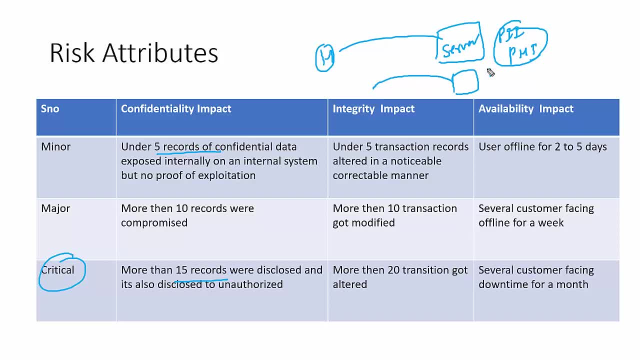 customer. Okay For me, if it's basically down for one hour, it has a big impact. If it's down for two hours, big, big impact. If it's down for five hours exceed my expectations. Okay, So we give the risk tolerance. 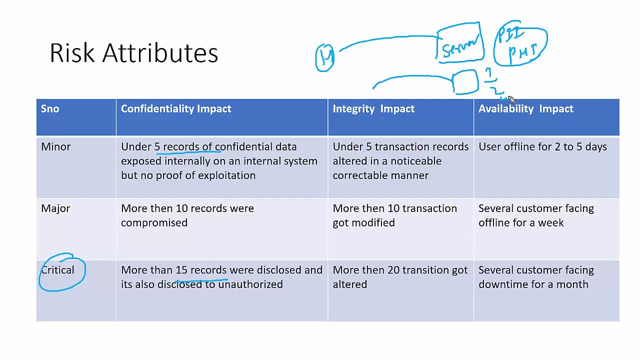 So we give the critical rating. So there's no data, So I cannot measure from a confidentiality point of view. So in this case confidentiality I will give cross, but availability I will make high, Integrity I will mention high, So sometime impact is organized based on a CIA. 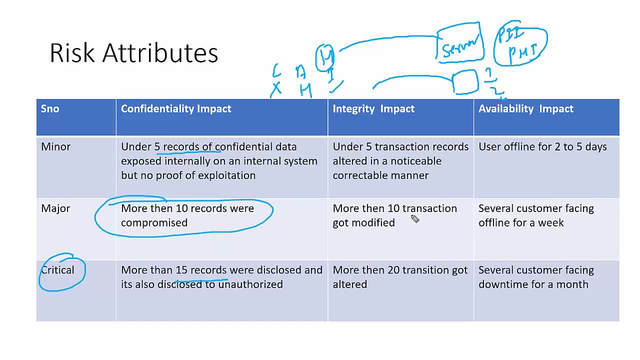 Now, here you can see, more than 10 record were compromised, more than 10 transactions modified, several customer facing offline for a week. So here the impact is basically varies from CIA trade. Okay, So this is the example. we have taken, the threat action. 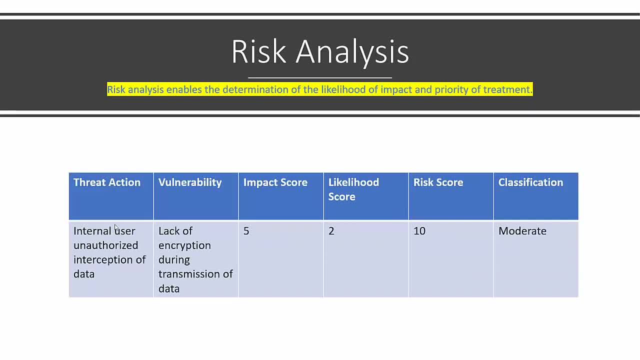 There is an internal user unauthorized interception of a data. What is the vulnerability? We have discovered the lack of encryption during a transmission of data. The question is: what is the likelihood of this threat action is going to exploit the vulnerability? Chances are two. 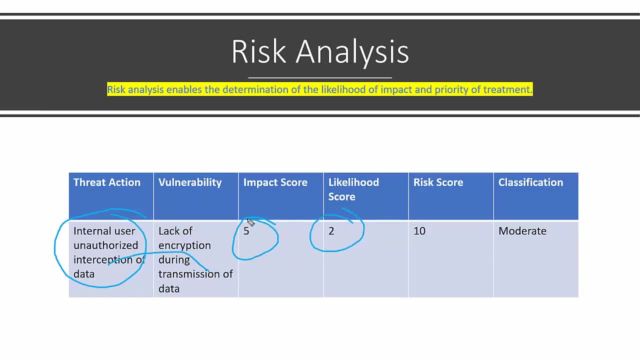 And this has happened. The impact score we have given is five because it basically disclosing a PI data, So five into two, 10, the classification we have given the moderate. it is just an example I'm giving Okay, So if you go to the same Excel sheet here, you can see the Excel sheet. 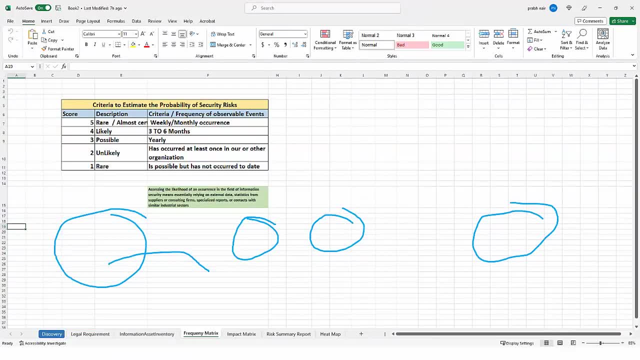 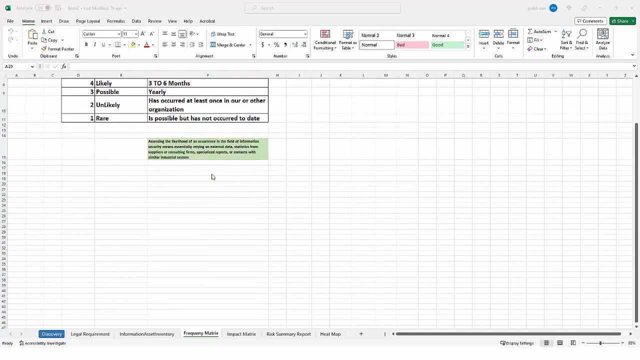 So we have categorized same thing here in the frequency metrics. So if you notice the frequency metrics, okay, frequency metrics is basically occurrence, So we have given the value is called: five is rare, Four is likely Okay. Three is possible Okay. 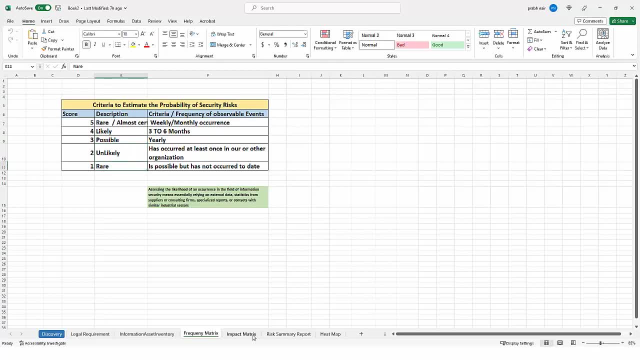 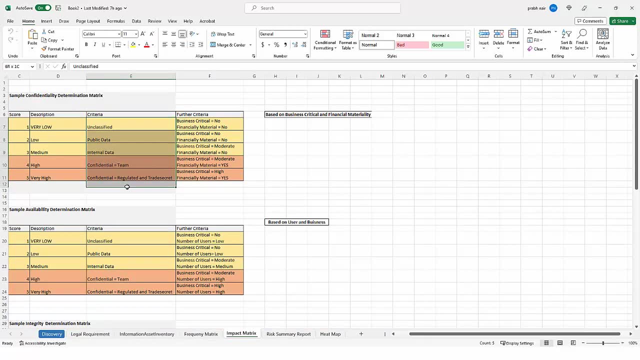 Two is unlikely, Rare, Okay, Based on a tolerance, And this is basically impact metrics. But if you see the impact metrics, we have a different, different type of impact metrics. Like we have a goal, We have a confidentiality impact metrics. 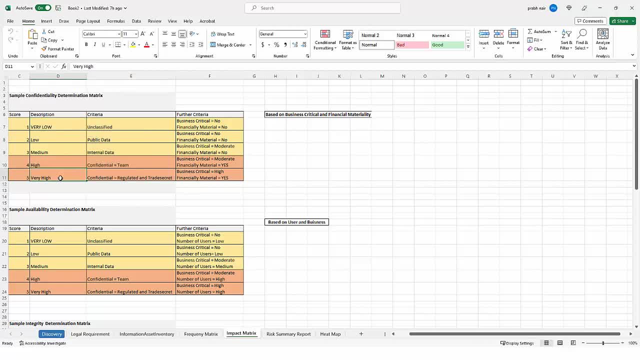 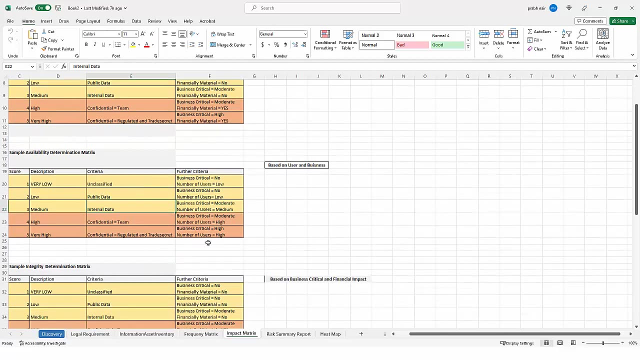 Okay, Here you can see description is very low but very high. in that case, the confidential data is regulated and trade secret. If regulated and trade secret data is basically compromised, business is critical, is high and impact is also high. Now, sometime we basically based on availability, vacancy here, based on our integrity, we have 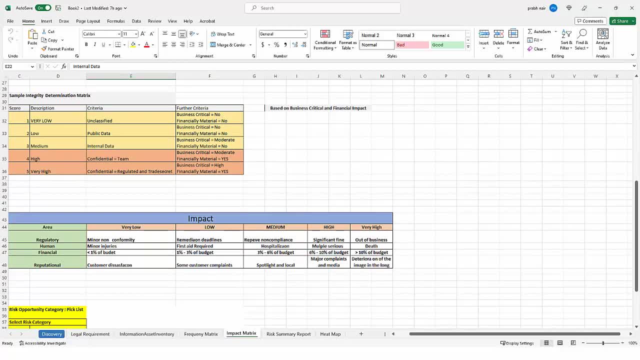 and this is how sometimes we don't have a CIA, So we give the impact based on a regulatory- Okay, We can give the impact based on regulatory, human, financial reputation. So it is. it depends, okay, how you basically define the thing. 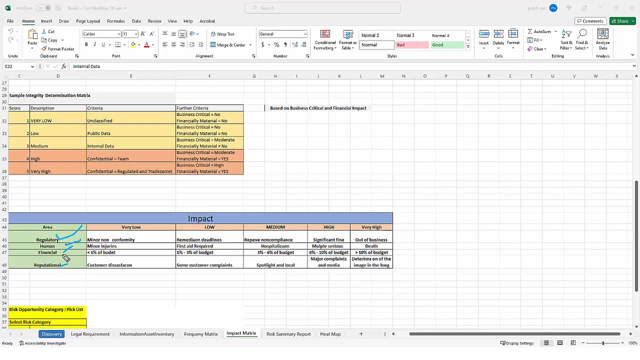 So in this case you can see there is a threat which is called virus basically attack the server. Okay, So there is a virus which basically attack the server and server is basically down the because of the confidential data. we need to answer to regulatory authority. 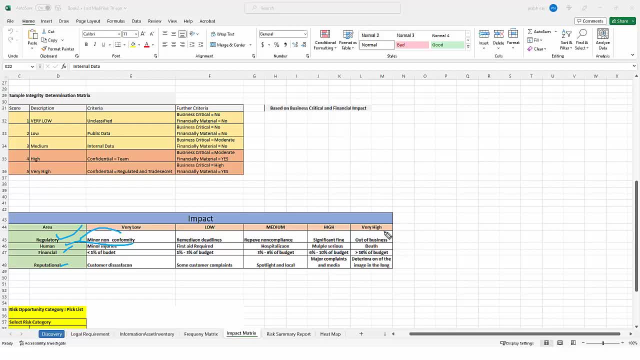 Regulatory has a big impact. So here we given: the very low is minor, but very high because it will might go out to business. Now same we have a physical safety. for that. We're doing a risk assessment. We discovered that suppression systems are basically unavailable. 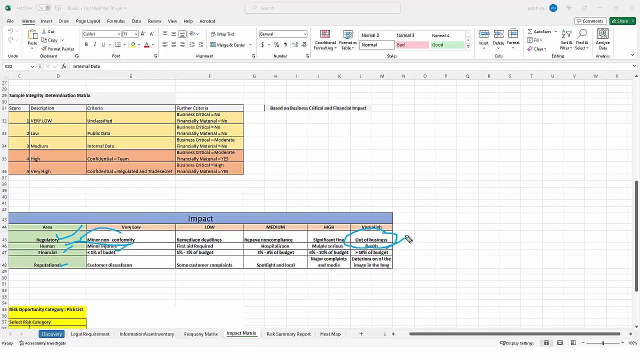 Minor injury very low, but major injury is basically death. So we know if suppression system is expired we need to replace that because impact is death. Okay, So sometime the impact is based on a CIA or sometime is based on these four dimensions. 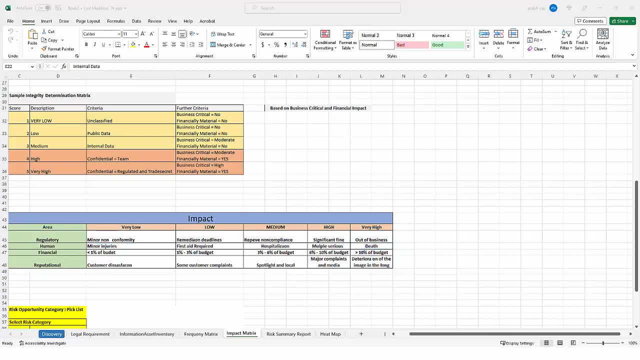 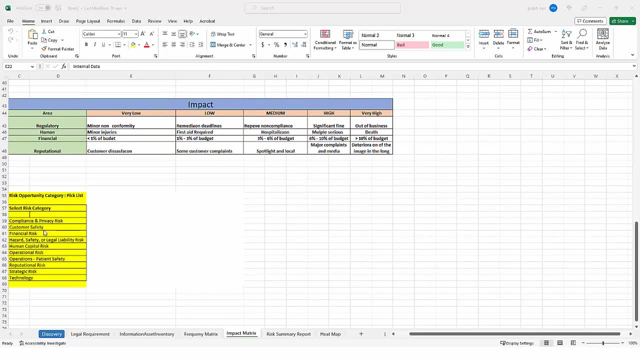 regulatory, human, financial and reputation. So it is up to your business How you define Here. We are recognizing a different type of risk category. Okay, Compliance risk, customer safety, financial risk hazard, human capital risk operation. 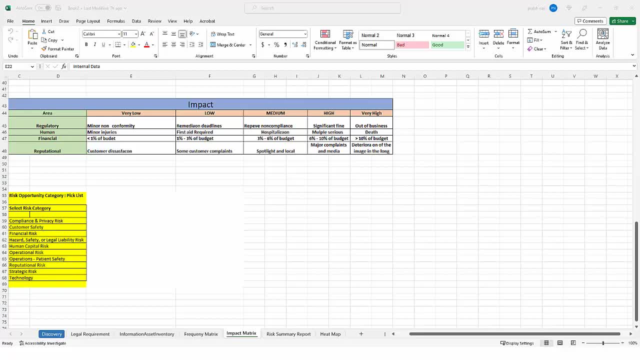 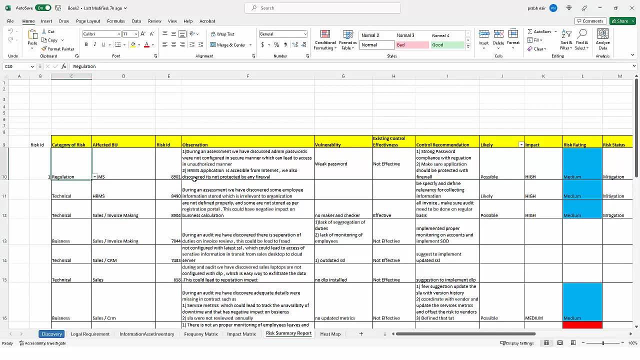 risk, operations, reputation, strategy, risk and technology. So that is how we have, And then, finally, we creating this risk summary report where we giving a category of risk. Suppose we have taken the example of my HRMS. So, category of risk, we have discovered regulation. 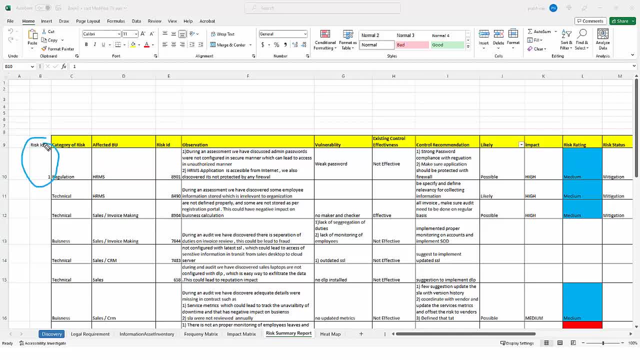 We have to give a risk ID because risk register will maintain that information. So category of risk is regulation. Affected business unit is HRMS Risk ID. We have given this 8,, 9,, 0,, 1, because that value goes to the common risk register. 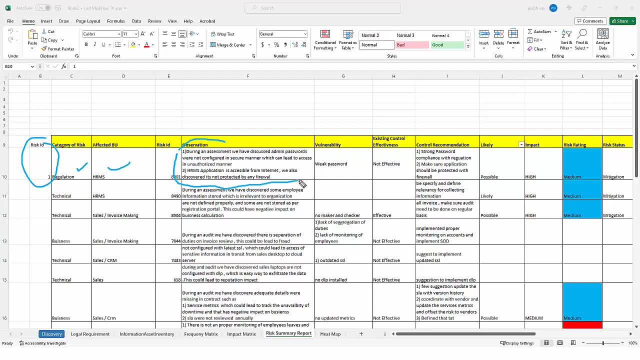 We have to explain our story and it should be explained in such a manner that it can be understandable to the person you know. during the assessment we have discussed, admin password were not configured in a secure manner which can lead to the access authorized manner. 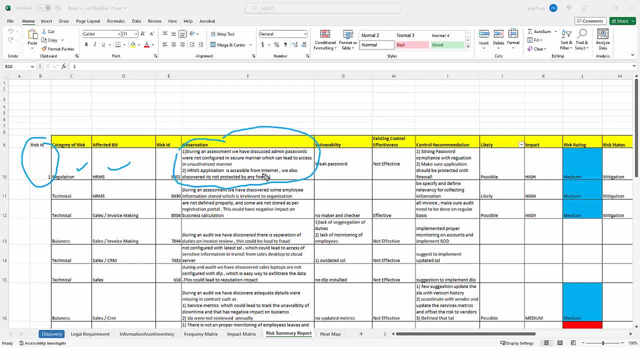 HRMS application is accessible from internet. We also discovered it is not correct by the firewall. So we just observing what we did, what we have seen and vulnerability we have discovered that is a weak password. Okay, There is a missing control. 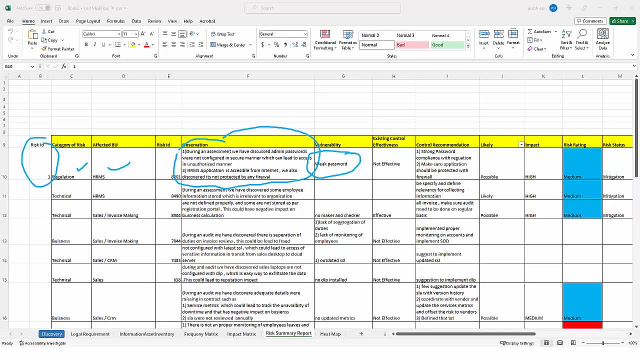 I could not find effective. There is was a control, but it is was not effective. Okay, Recommendation is: control passwords. Make sure application should be protect from the firewall. Now, likelihood of of this HRMS going to be exploit: likelihood: 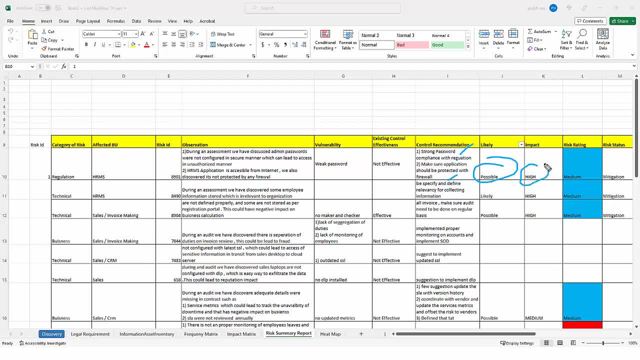 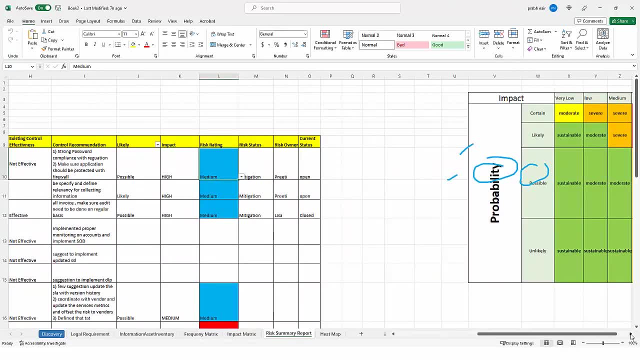 I give the possible okay And impact is basically high. The reason why the HRMS basically store the employee data. That's why the risk rating I given the medium. now from where I got this value, because I'm sure this is a question. 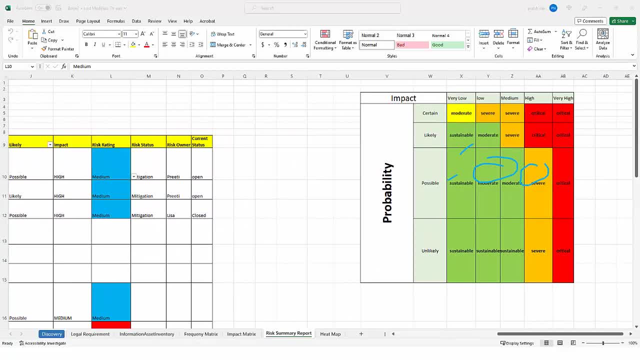 So this is how the metrics we create. So if the value- suppose we have a value called likely and the impact I basically mentioned, high, So in that case the risk rating will be critical If I say the impact is basically possible. 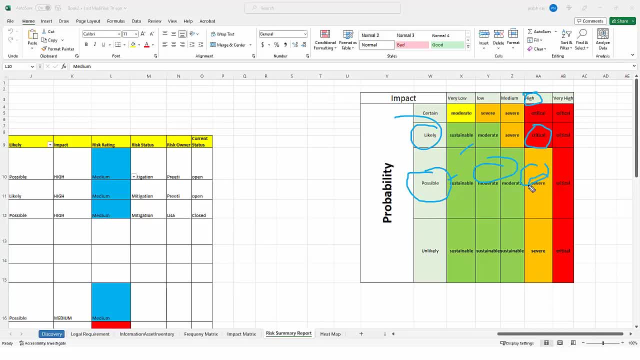 Okay, Sorry, Probability is basically possible And impact is basically severe. Okay, And from where I get this value? based on a CIA regulatory reputation and all that. So I will basically give the value risk rating here. Current risk status is mitigated. who mitigate it will be by Lisa. 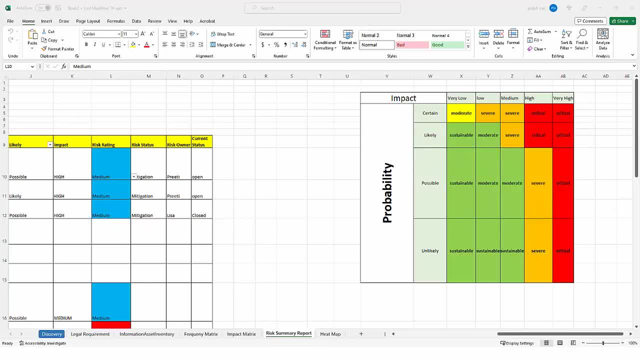 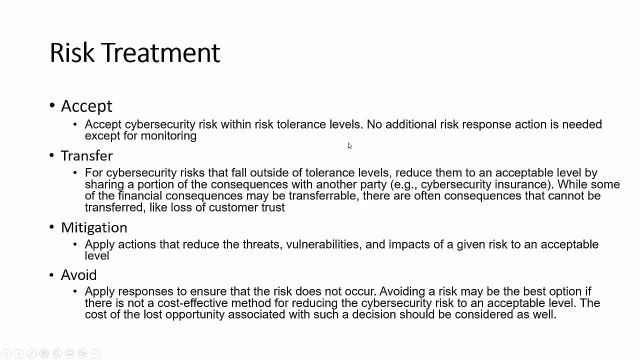 Current status is basically close. So this is how we basically give the value. Okay, Coming back to the slide, When we talking about the treatment, we have a four type of treatment, except the risk: transfer the risk, mitigate the risk and avoid the risk. 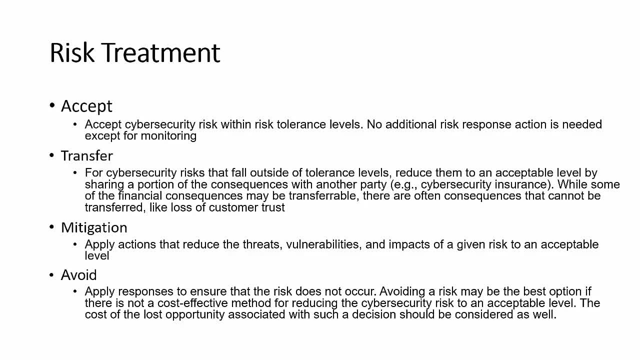 So we accept the risk in that case. when the risk is below the appetite: okay. Below the tolerance level, or the cost of opportunities higher than cost of risk: Okay. When the cost of control is higher than the cost of risk, we know it doesn't make sense. 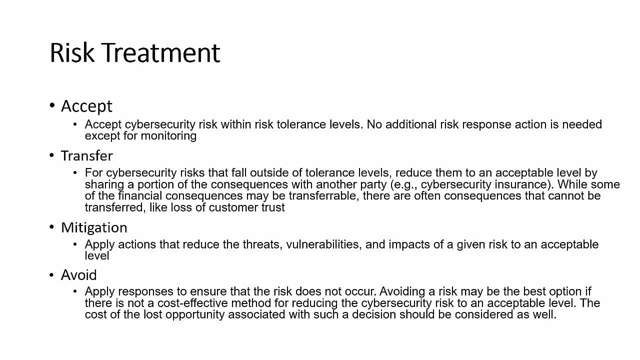 to implement the controls. In that case we accept the risk. Okay. Second, is we transfer the risk? We transfer the risk to third party. We basically transfer the risk in that case when likelihood is low but impact is high. We know by the cyber insurance we can buy the risk. 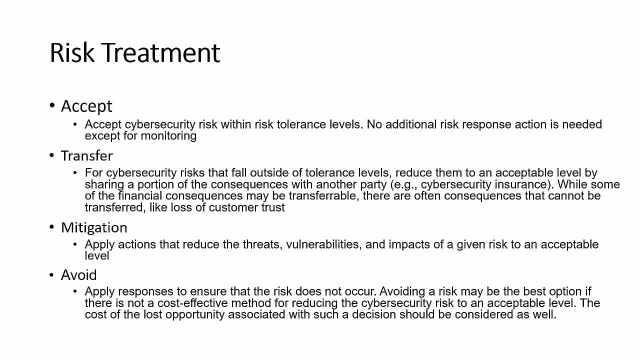 Third is we basically mitigate the risk by implementing control And after the risk which is left more normally, we go to accept. And last is basically called as a risk avoidance. Risk avoidance basically mean we avoiding the opportunity, We avoiding the source. 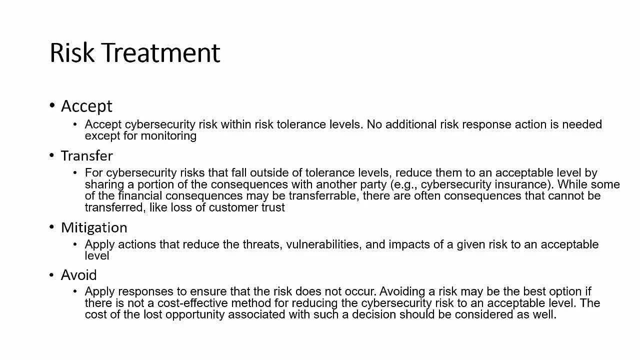 We avoiding the source which bring risk to the organization. Okay. So example like discontinuing one application, not giving CSSP exam, is like avoidance of risk. Okay, So avoidance risk may be the business call, but acceptance risk is basically the IT call. 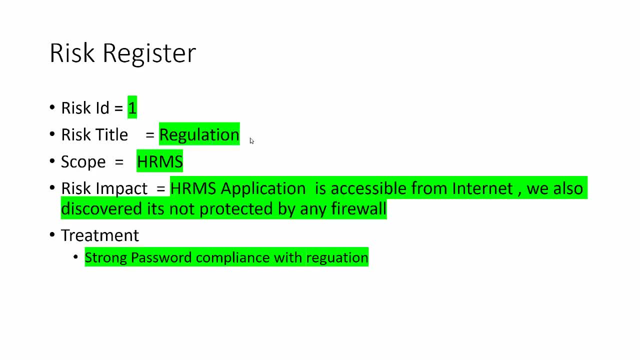 Okay, That's the most important thing. So when we documenting everything, we are creating a risk register in which we maintain the risk ID. Okay, So this is supposed risk ID when I given. So if you take a reference of the Excel sheet, this is basically called as a risk ID. 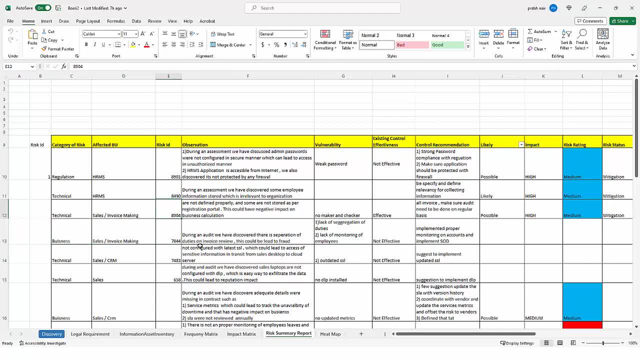 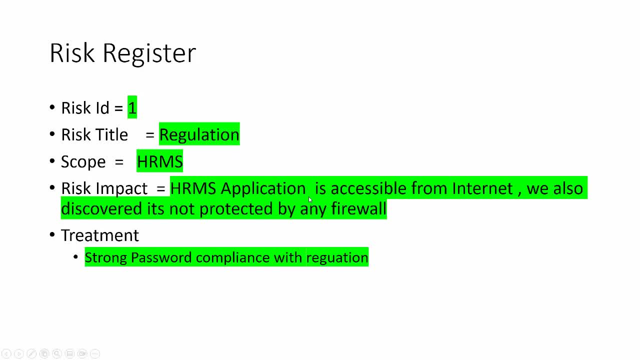 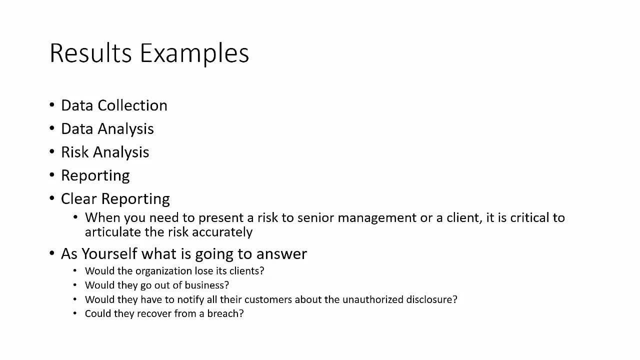 Okay, So risk ID is basically, suppose 8904, risk title is regulation, Scope is basically HRMS. Then we explaining about risk impact and what is the treatment we have suggested. When we talking about the results, Okay, Okay, In the result we consider different kind of data. 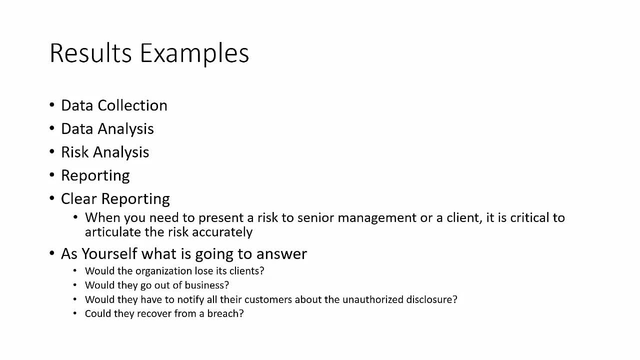 Okay, So we need to have first data collection document request list Like example, like they will we need to have when you presenting the reports finding to the management. Okay, We need to have some set of documentation. So in the data collection, the first part we need to have is records of interview asset. 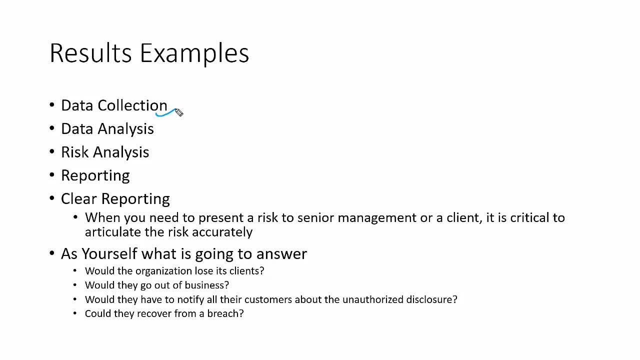 inventories, you know, asset listings, what the assessment you did right. Then contact list. Then we have a data analysis. It mean the issues, observations, okay, Threat, catalog vulnerability, catalog control analysis, risks, or then risk analysis basically. 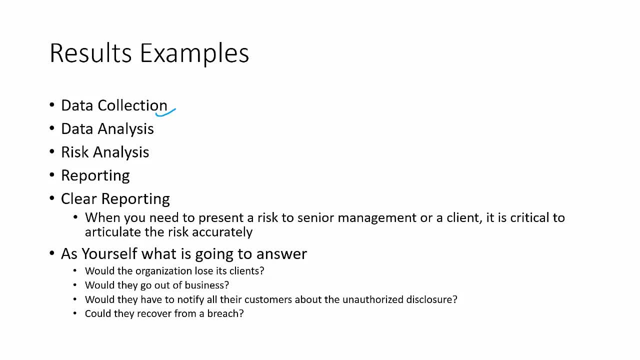 all about your risk categorization metrics and finally, report. So these are the documents you have to maintain. Okay, So, when you preparing a report, there is a most important thing is that when you need to present risk to the senior management or a client, it is critical to articulate the 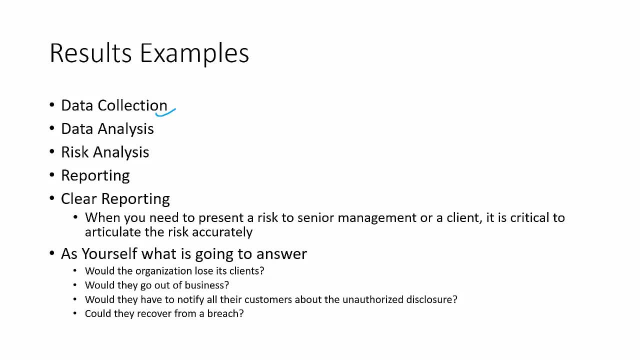 risk accurately. So when you basically presenting something- okay, suppose finding, and all that, one thing we need to understand- when you narrate the finding, ask yourself, ask yourself, would this organization lose it client, Would they go out of business? 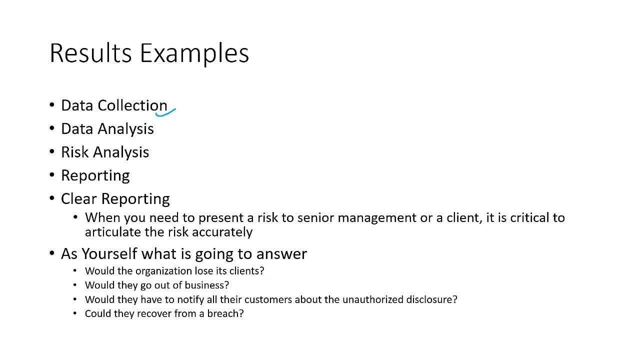 If we don't mitigate this, would they have to notify all the customer about the unauthorized disclosure? Would they recover from a beach? So if your risk description does not answer these questions, then you have not fully covered the component of a risk. How? let me give an example. 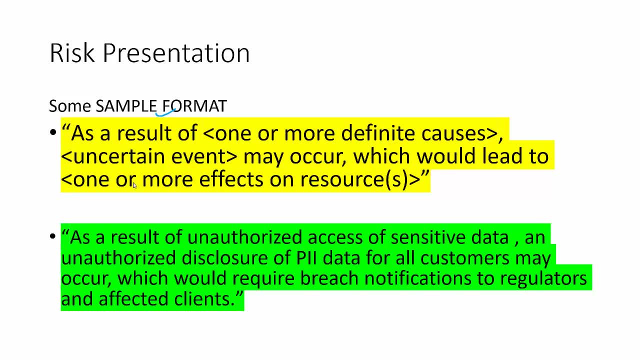 See: as a result of one or more defined cause, uncertain event may cause which would lead to one or more effect on the result. This is the template we have. Okay, So I've given the reference. as a result of unauthorized sensor data. 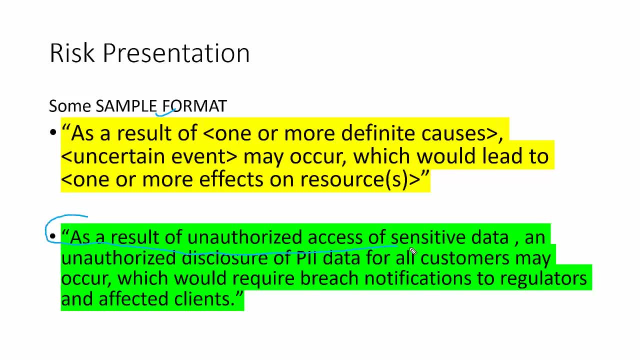 So this statement I have basically used as a overall outcome. as a result of the unauthorized sensor data, Unauthorized disclosure of PI data for all customers may occur, which is called as an event Okay, which would require the brief notification to regulatory affected clients. 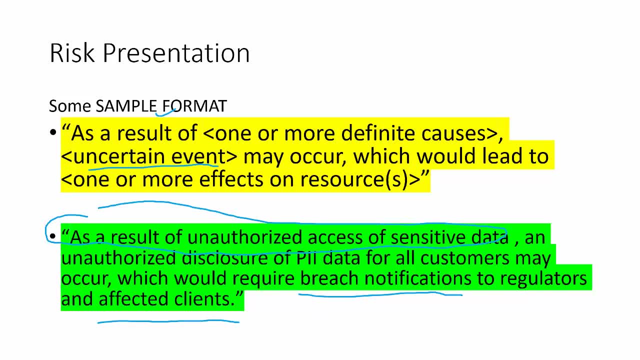 So it means we need to notify the regulators. So it is easy to confuse the threat and vulnerability with the risk itself. Okay, but think of a risk as a description of the consequences. What would happen if the vulnerability were exploited? Remember risk details, the impact to the organization. 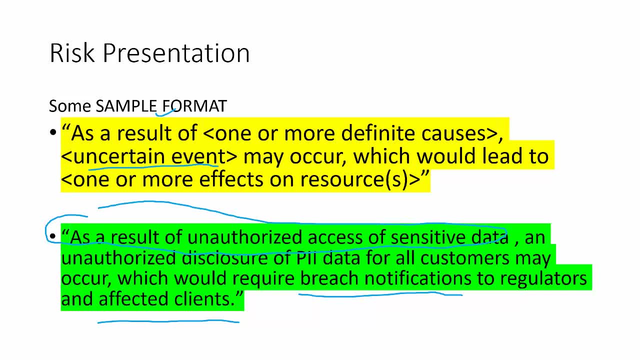 So your statement, your value of clear and concise communication cannot be overstated in the risk management Okay. so no matter how accurate your risk model or how thoroughly your threat analysis, it will be definitely meaningless if you can't effectively present to the business.